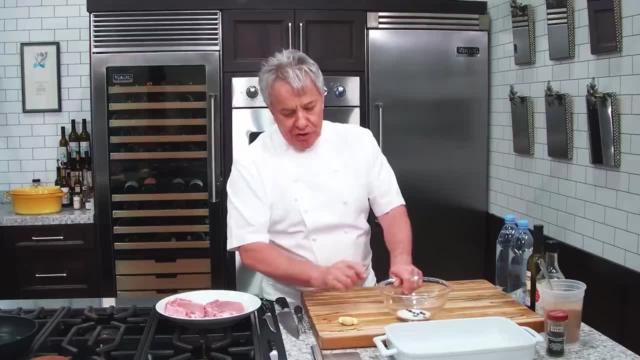 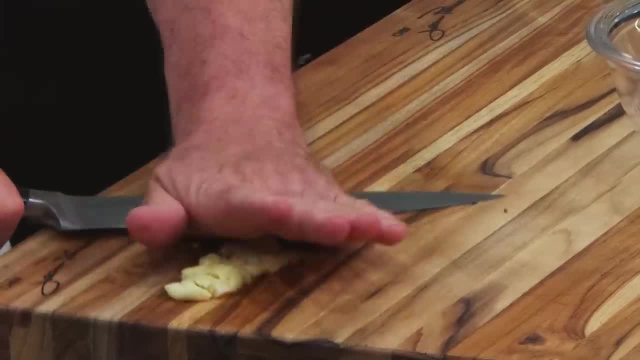 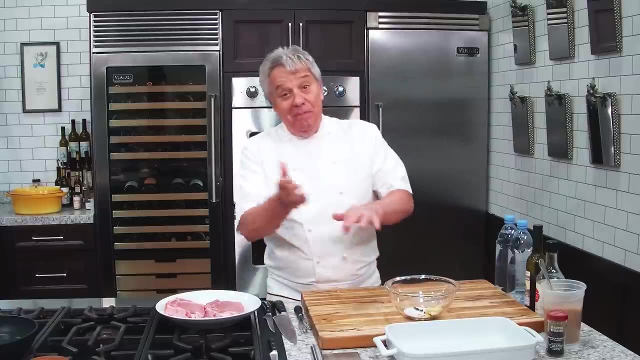 going to put this with. I got about two tablespoons of salt right here that I'm going to mix with about a quart of water, roughly maybe a little bit more. I got some garlic cloves. Like I said, the flavor of it very little is going to get in. Now we're going to get a little bit of a flavor. 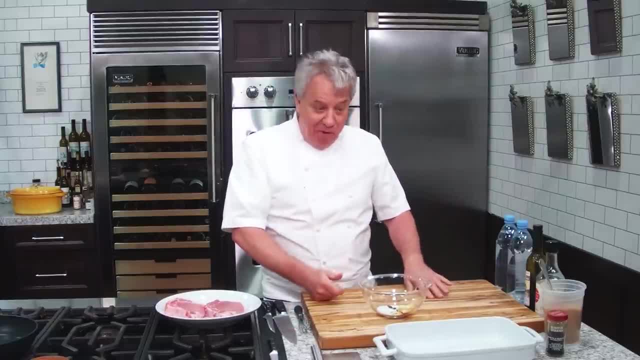 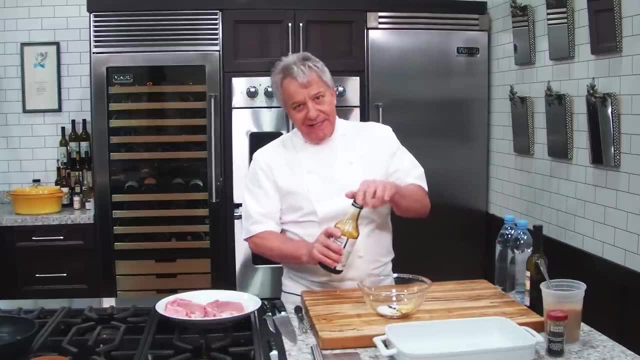 water. Some of them is going to get in because the water is going to get in to the pork. So we're going to get some of that. flavor is going to get in there. Also, I put a little bit of soy sauce because that's going to be really an introduction of salt Again. it's going to help us So a little. 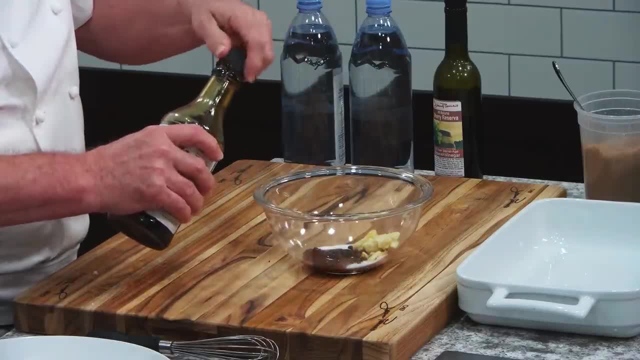 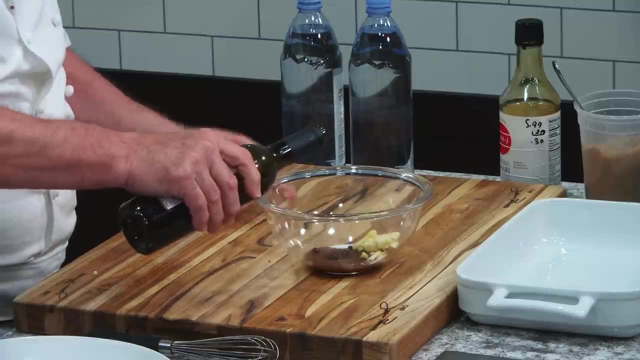 bit of soy sauce. We don't need a lot. What would you say A large healthy tablespoon? I'm also going to put a little bit of vinegar. I use it. I like to use for the pork a sherry vinegar I got. 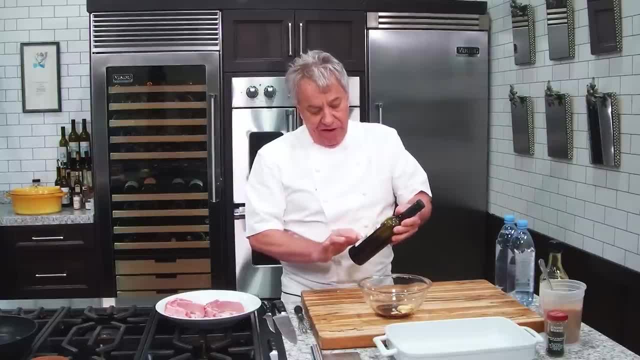 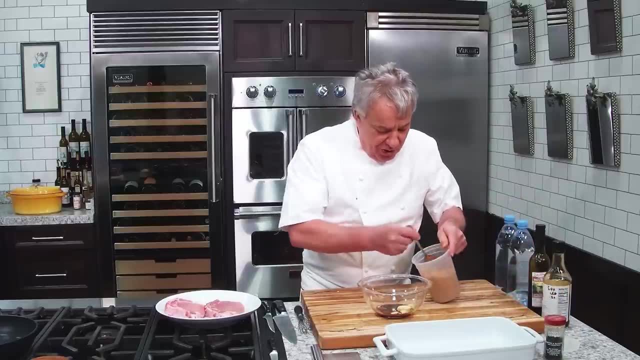 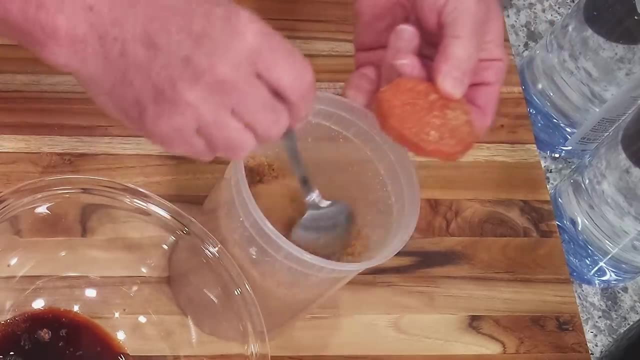 this beautiful sherry vinegar. This is a 25-year-old Spanish sherry vinegar. It's beautiful. I'm going to put it in here. I got to put a little bit of sugar. Oh, you know, I keep forgetting to tell you about this thing, This thing right there. Keep my sugar. See, look, it's not sticking My. 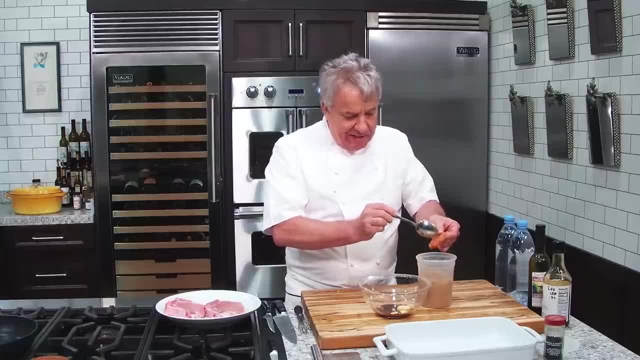 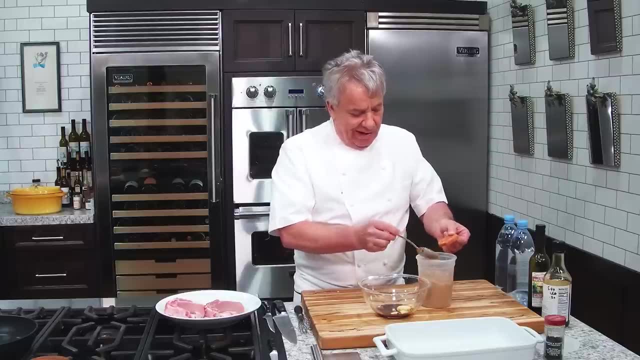 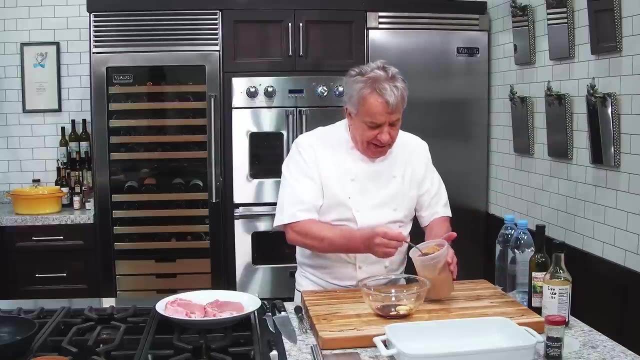 sugar is not sticking at all, And it's because of this stone right there that is made out of clay, And so I said, well, I don't have any one of those, I'm going to break one of my clay pot and put it in there. It didn't work. Somehow this thing worked. I don't know how it. 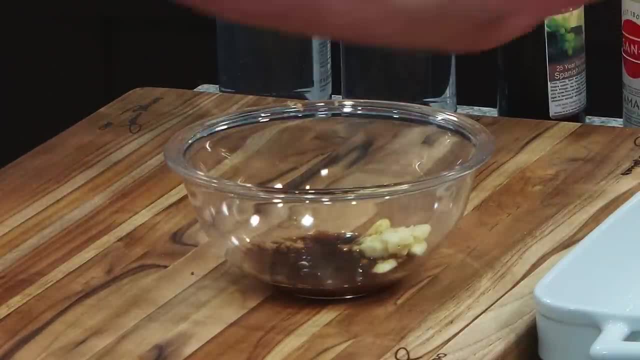 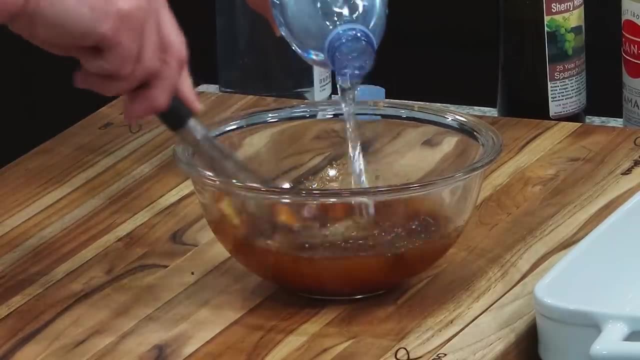 works. So I'm going to put a tablespoon of sugar and I'm using a brown sugar, light brown sugar. I'm going to mix all this up and I'm going to put some water friends, And this is about a liter of water right there. We're going to mix all this up. really good, We're going to put it in. 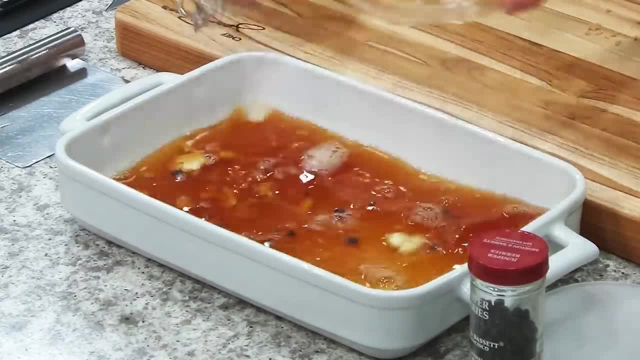 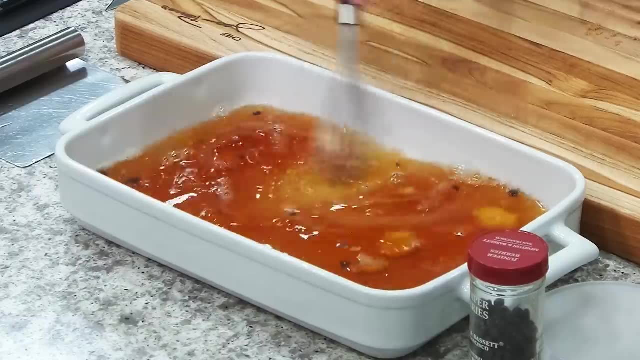 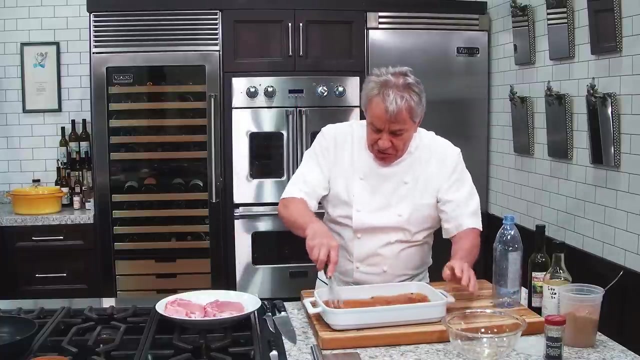 here and right in there. Really simple. I'm going to finish the whole bottle, Probably going to need it all. The secret is to make sure your pork chop are solid. You know, I do the same thing with my pork- pork loin or pork tenderloin, Same deal. You can do it in a Ziploc bag. Make sure the salt. 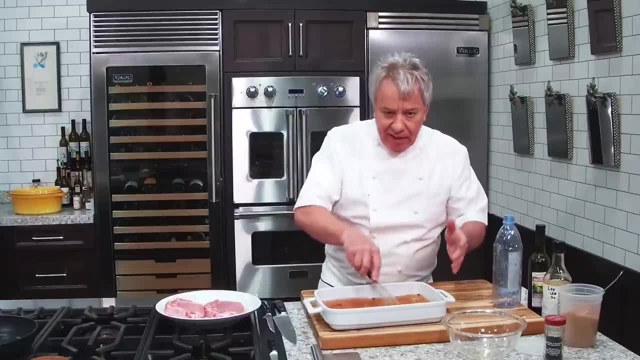 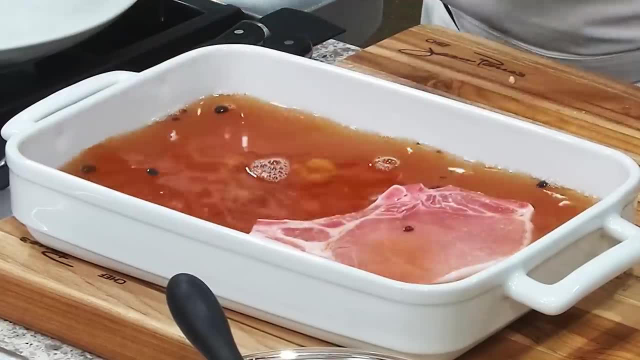 is well dissolved. It's very important. You may want to take a little more time dissolving it there, Right? And then you're going to take your pork chop- I got some beautiful rib chops right there- And bone in You can do, bone out, You can do whatever you want. The secret now is to make 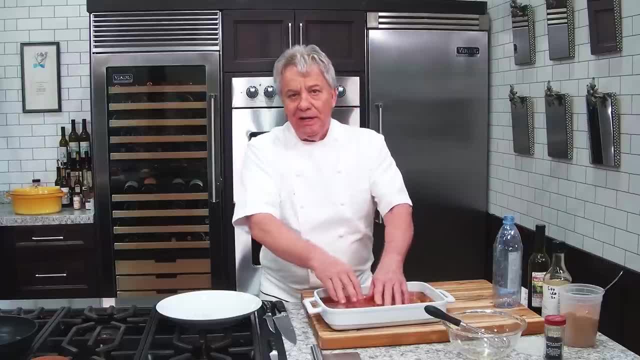 sure we put a plastic film on top of this, unless you do it in a Ziploc bag. Remove all the air and you're good to go in the bag. Otherwise I'm going to put it in here And then I'm going to. 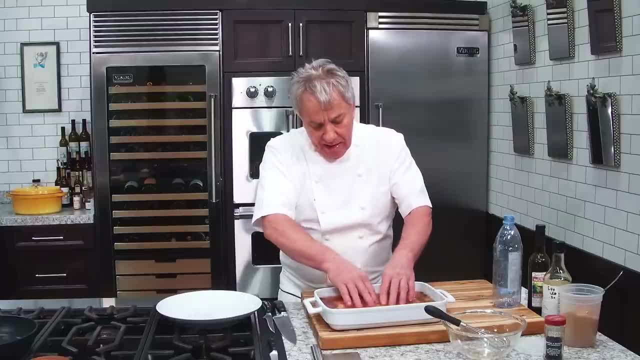 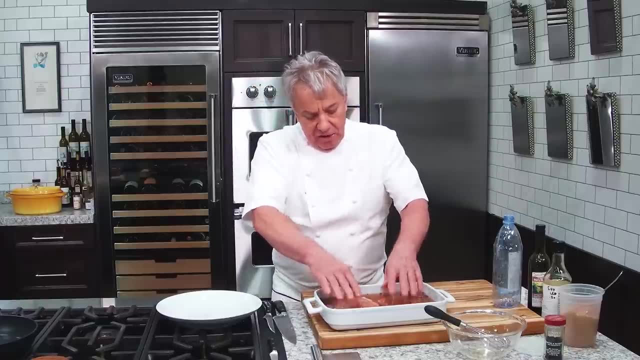 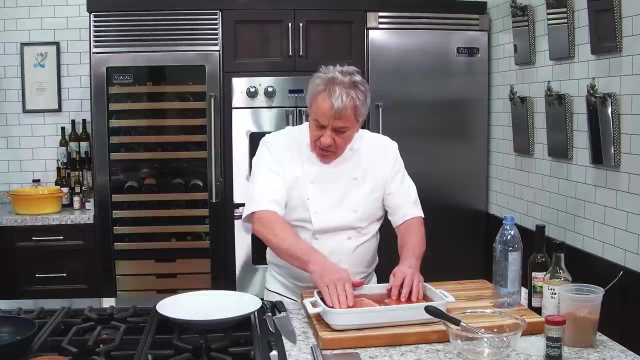 put my plastic right on top of this And I let it. How long do you let it go? No more than six to eight hours. Six to eight hours And you're perfectly fine. So we're going to wait for the six hours. We're going to wait six hours- I like to do six hours- And then we're going to cook it. 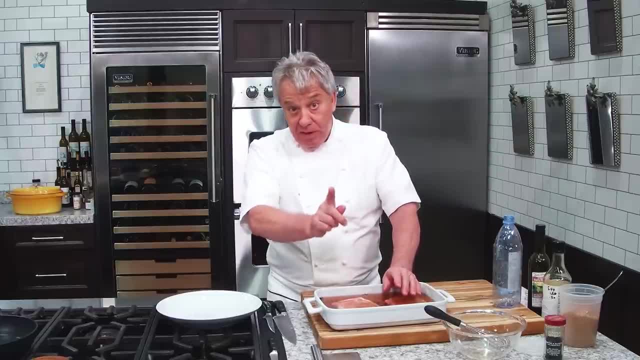 together. All right, friends, So we'll be back. I'm going to put them in the fridge, You put them in the fridge And I'll be back in six hours, But for you it'll be just in a flash, Okay, friends. 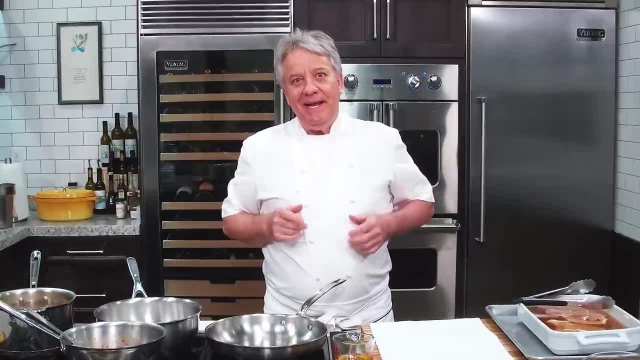 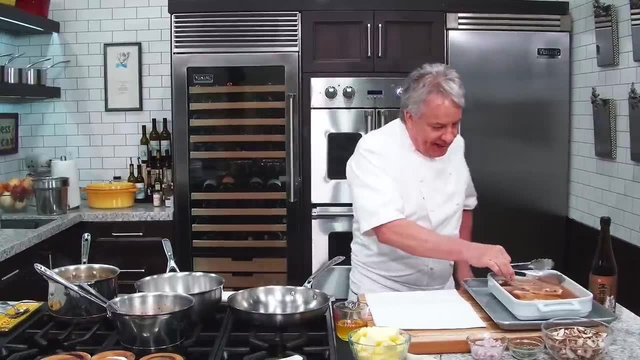 Pork chop have been marinated, Not marinated. I'll start again. Okay, friends, Pork chop have been brined, They're ready to go, And we're going to take them out of the salty water And we're going to dry them really. 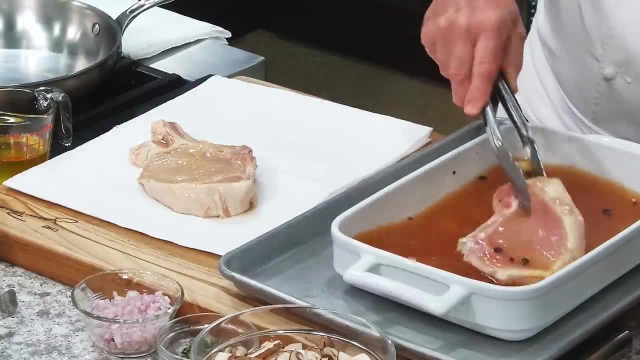 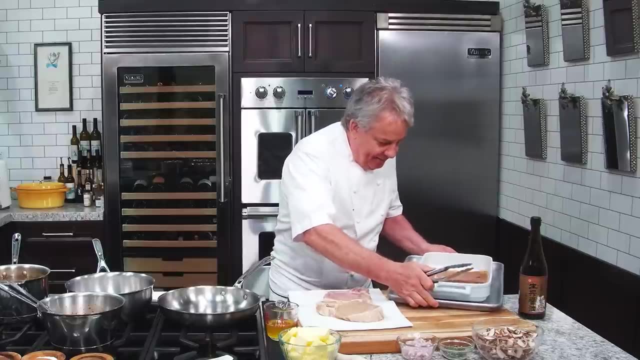 really good, And then we're going to saute them. Now, one quick little thing we got to do, And don't let me forget it, I got to. first. I got to get rid of this. I got to, I got to make a couple of things. I got to make a couple of things. I got to make a couple of. 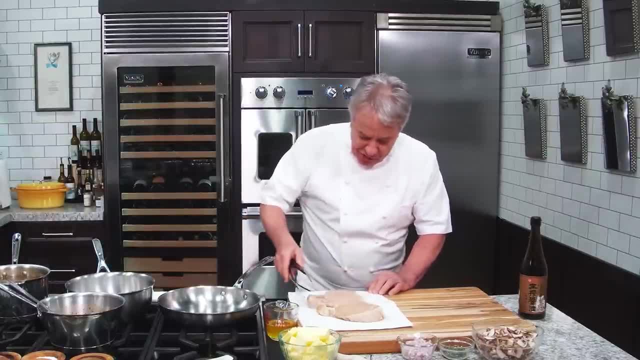 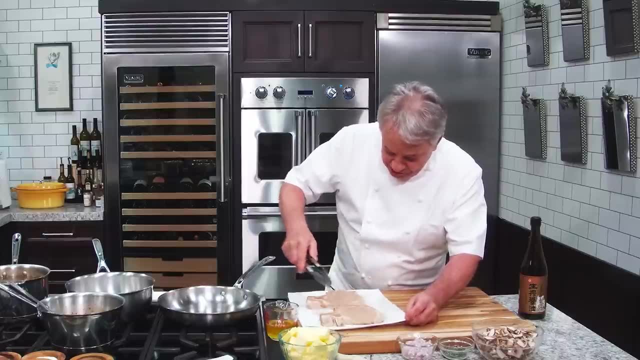 slits in the fat so they don't shrink on me. I'll show you what I'm talking about in a minute. Actually, this fat cap is pretty good, So I don't think it's going to have any issue. But let's, they look kind of strange, don't they? But they're not. This looks better than this Same. 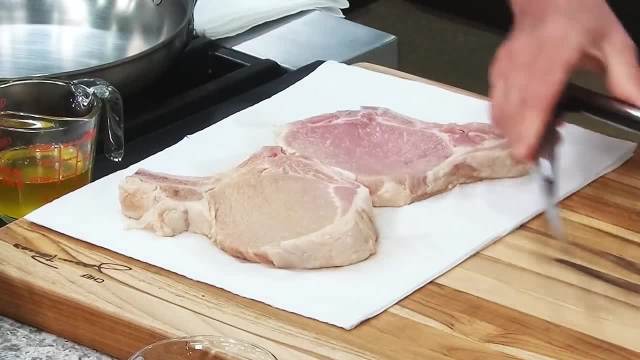 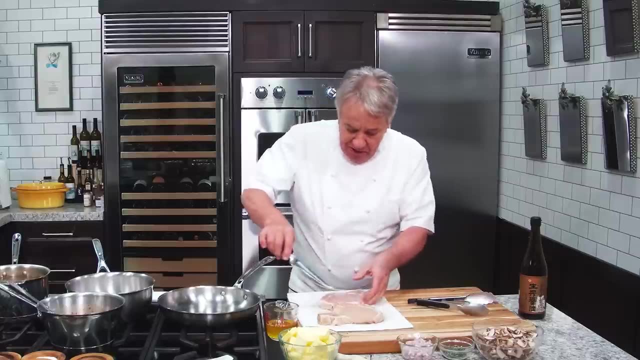 thing really. So we want to just take a knife right there, friends, And a boning knife would do just fine. Now, normally you got a big fat cap all the way around. You don't have any Otherwise. you just give it a little slit right there. You see, You give it a. 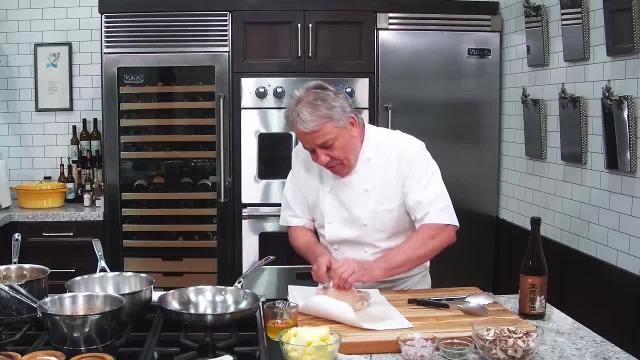 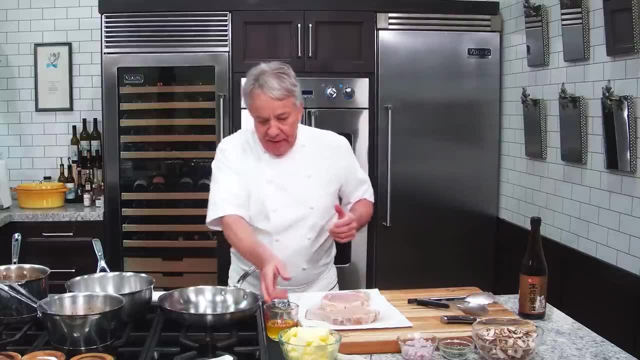 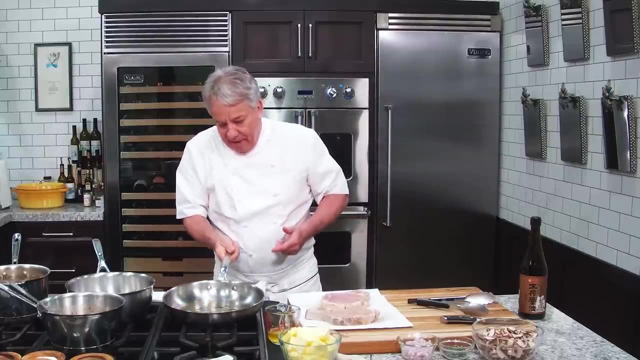 little slit about every two inches or something That avoids the fat from shrinking it, so they won't be very flat. And then they don't. they don't seal pretty well in the pan. You'll see, Just when you have a big fat cap. this one doesn't have any, So it's not that big over there really. 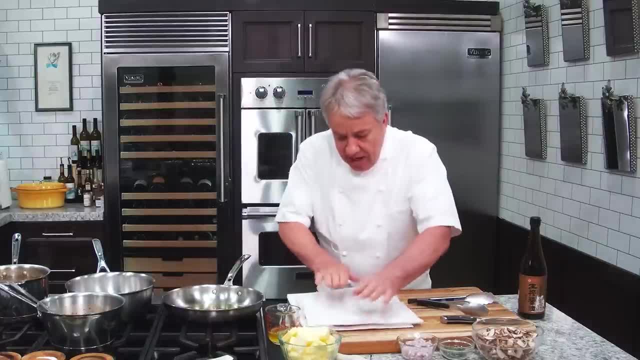 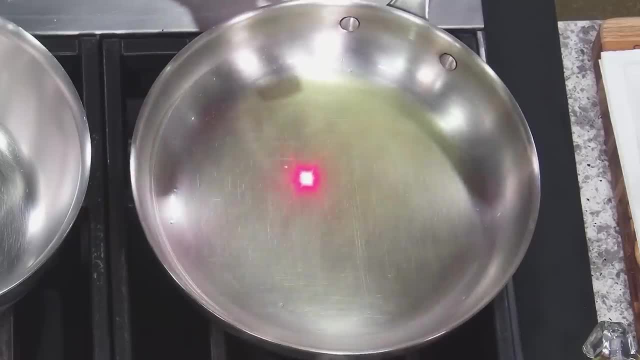 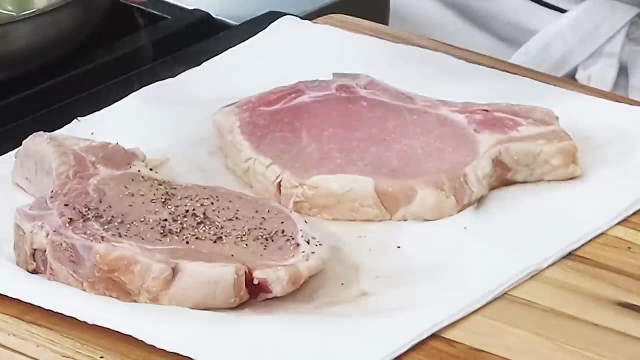 So I made a big deal over nothing for these guys right there. They're going to be nice, You watch. So I got clarified butter, friends, And it's ready. So I better move. My clarified butter is ready. I'm going to put some black pepper in there. You know I like a very coarse. 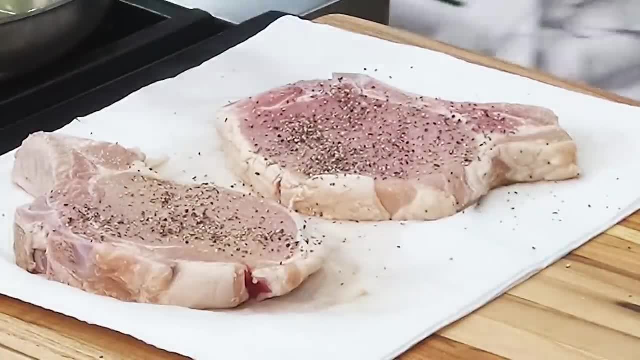 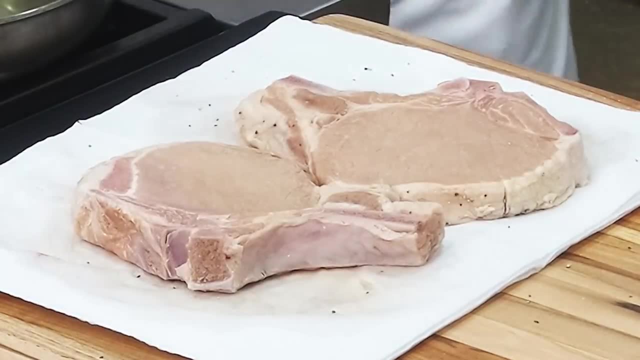 black pepper Salt. we're going to go very light because we already got salt in the brine, so we don't need it. And at one side, that was enough. right there, friends, And we are now going to put them in there. 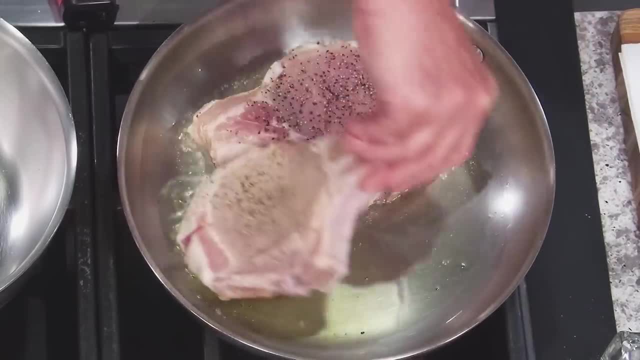 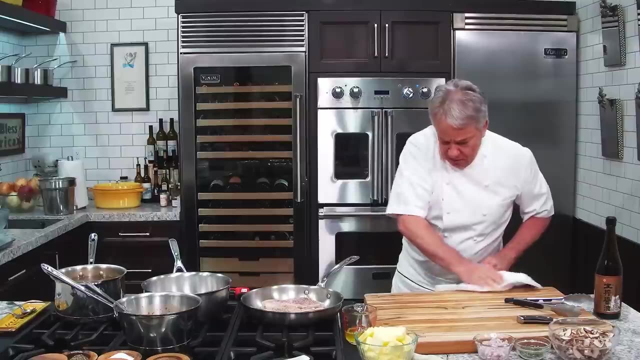 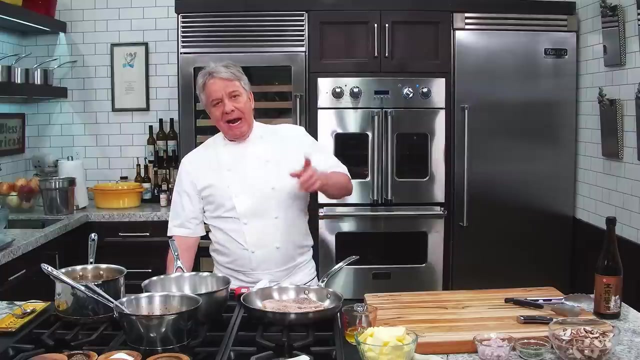 And we're going to leave them alone. Leave them alone for a second to get some beautiful Maillard reaction, caramelization of protein. Okay, friends, Going to leave them alone. Now. you can do it in a pan if they're very thin, But when they're quite thick like this, you know I like to pop them in. 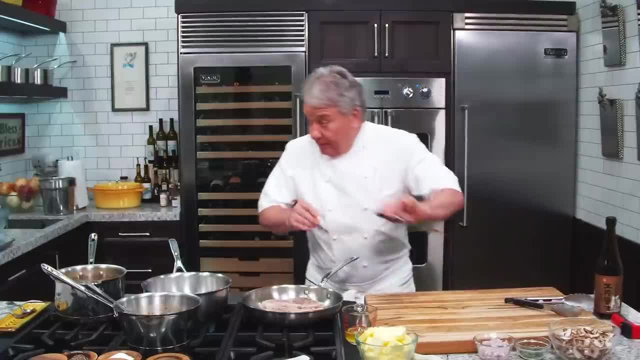 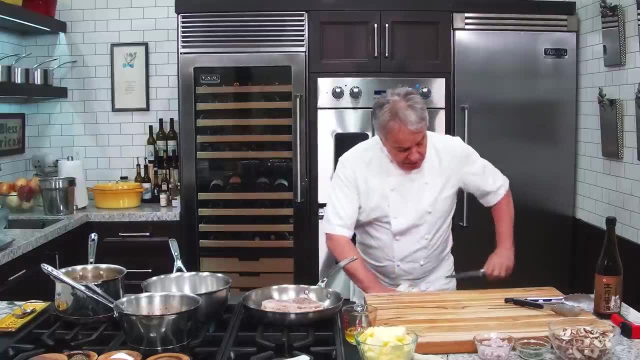 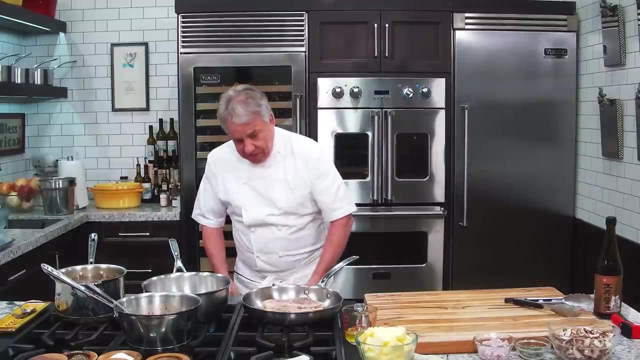 the oven for a few minutes. That's what we're going to do. And now the secret. let me clean this up. Besides the fact that we don't want to overcook them, we, we, really. oh, hey, look, come back over here see how you turn it off for a second. 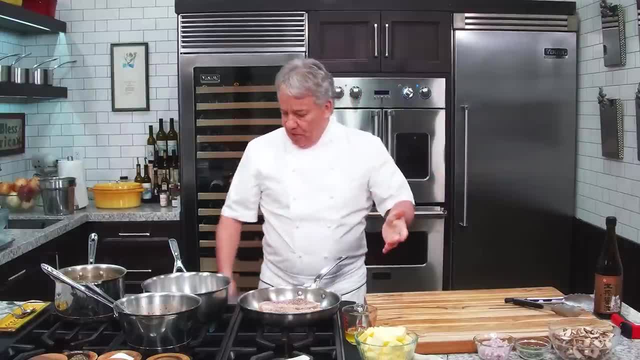 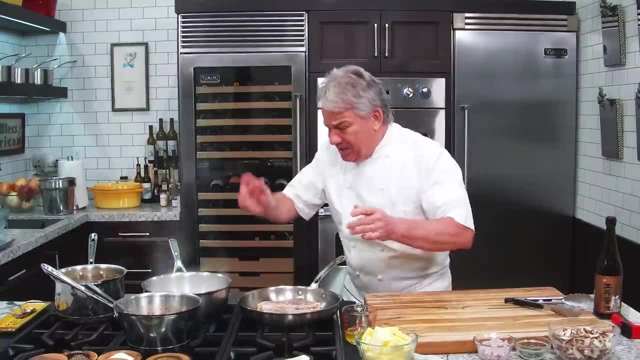 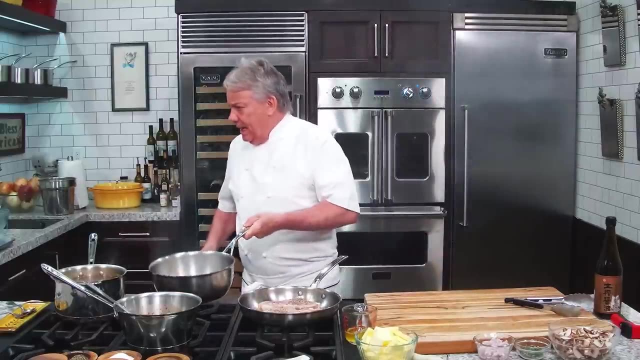 i don't want to overcook, let's put it that way. i, the most important thing is, i do not want to overcook it. and pork. a lot of people cook pork like at 150, 165. oh, mama mia, this is very hot too. this is very hot, very hot, very hot, a little too hot. that's what happened when, like you do, like tv. 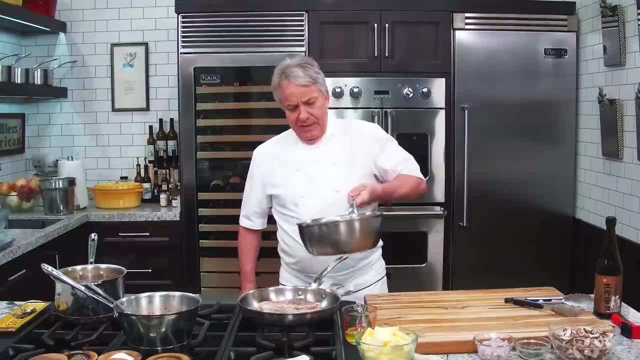 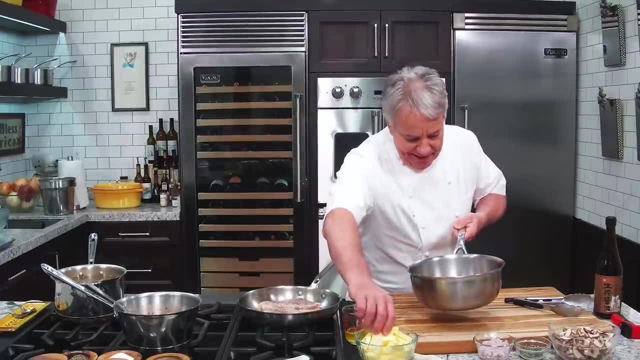 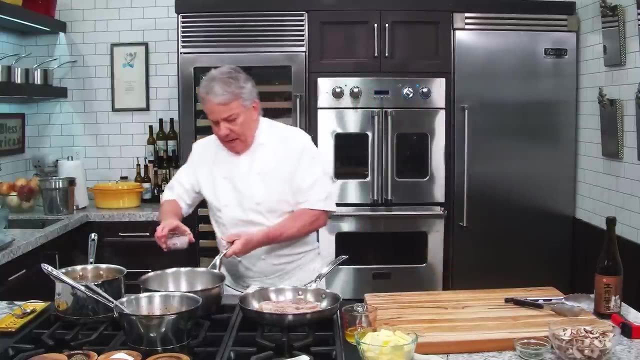 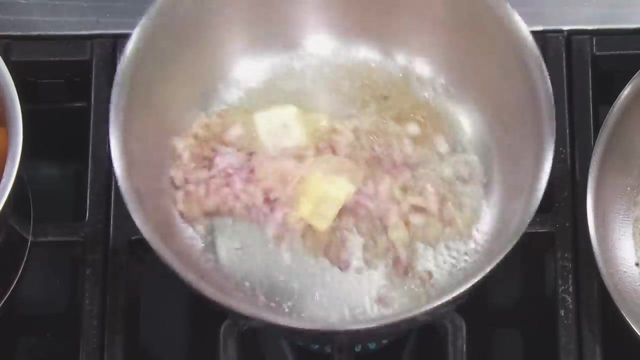 folks, folks, you see what happened. i burned the butter. that's okay. you know what it did. it helped me. it's like nice brown butter. it helped me. um uh, seal the pan right there. so here we go: little butter, reduce the heat. that's what happened. when you do live tv, you get the pan ready and they get. 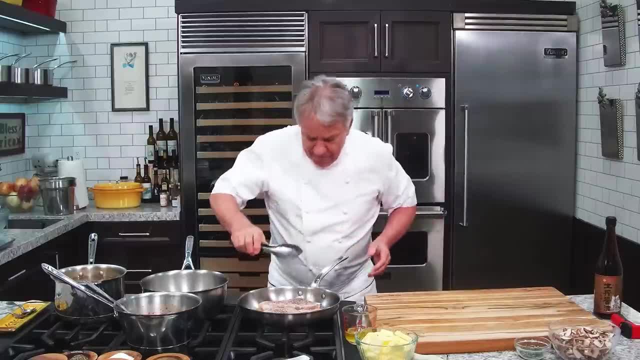 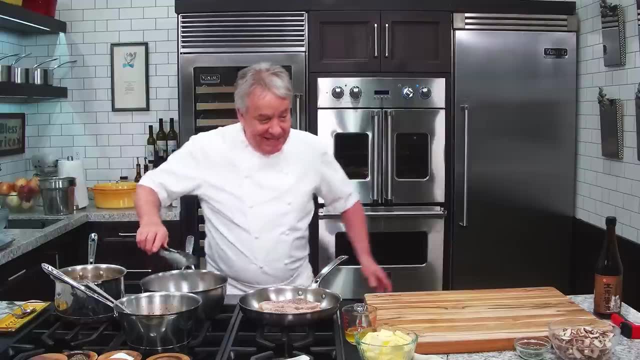 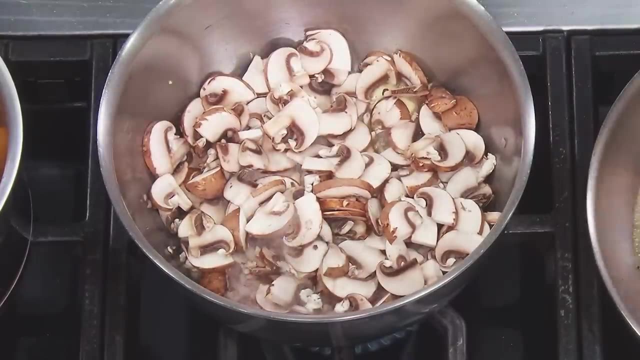 too hot. um, i forgot what i was going to talk about, um, because this got me distracted, so. so this is going to be a really nice, easy sauce. folks, we're going to make a little sage mushroom sauce and we're going to put the ingredients in that sauce. 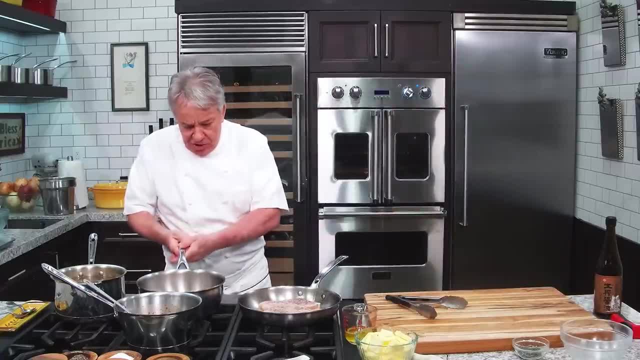 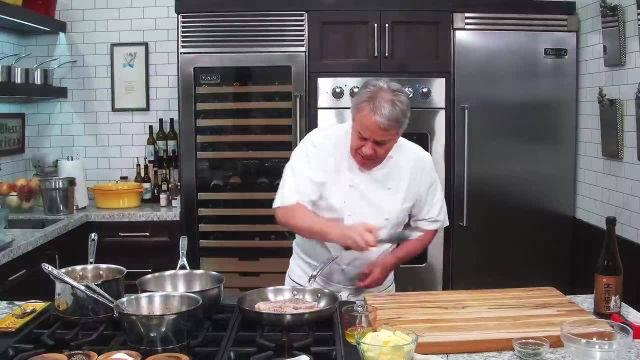 they're not familiar to this dish and uh, so we're going to put a little pepper, a little salt in there and how we're doing over there folks, like i said, if it's small, if they're very small, you can probably do them in a fry pan. 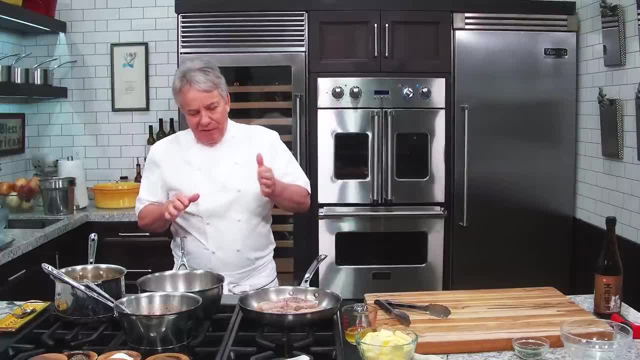 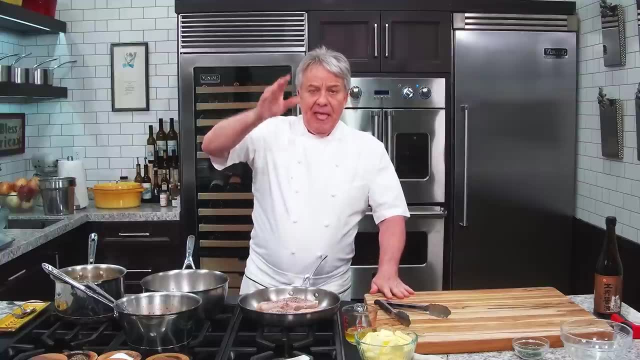 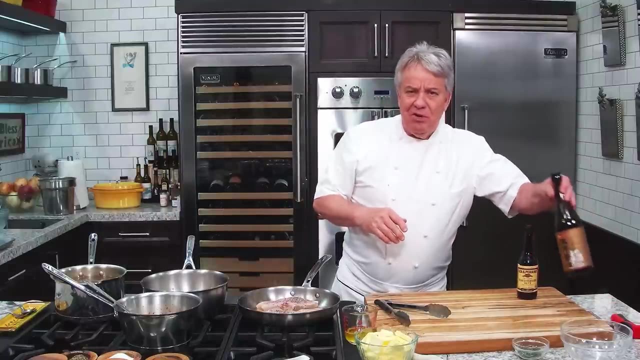 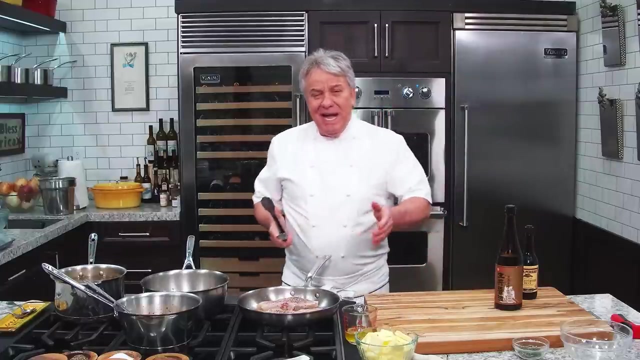 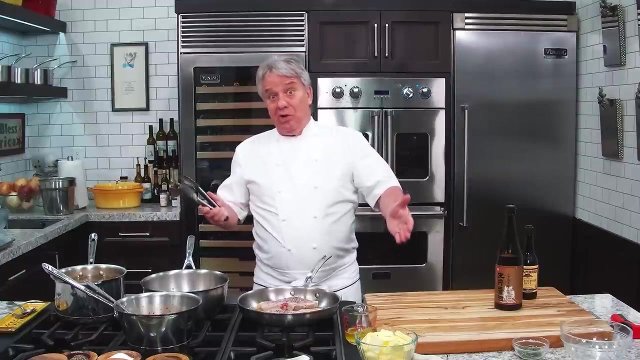 the first thing i just want to shout out: toasure здесь pour la item on your opening to make sure that the garlic is cornatiques a. If you're afraid of it, don't worry about it, As long as you cook it at 138 degrees. 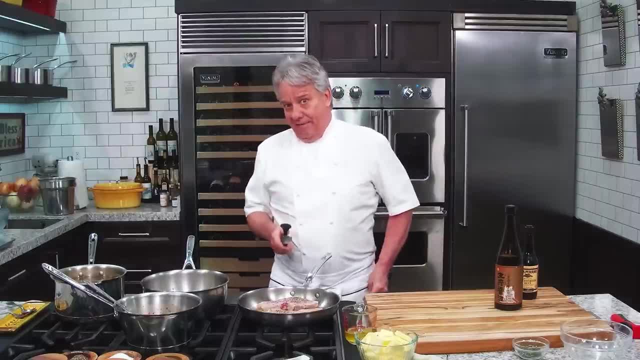 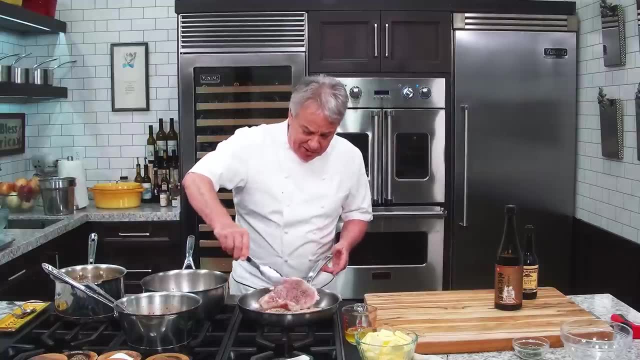 that's actually to not cook enough for me. I like it 145,, 145,, 150.. Oh yeah, I like it slightly moist, slightly pink in color. This is gonna be fine, probably in a fry pan the whole time. Now we're gonna make a little sweet potatoes mash. 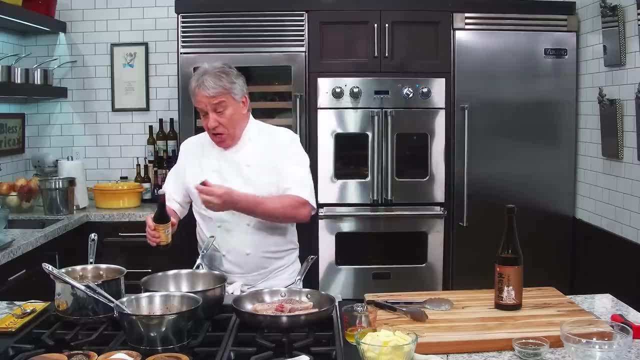 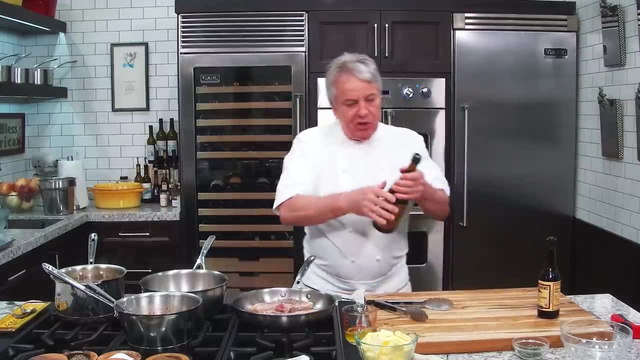 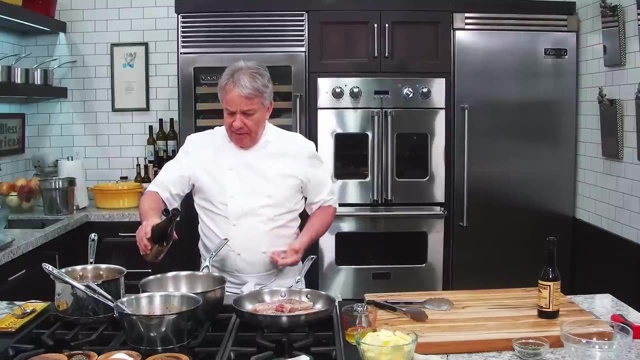 I use it in a few recipe, but I never showed you how to do it from scratch, So I'm gonna show you today. I put a little bit of a Worcestershire sauce And then, since we put a little soy sauce in the brining liquid. 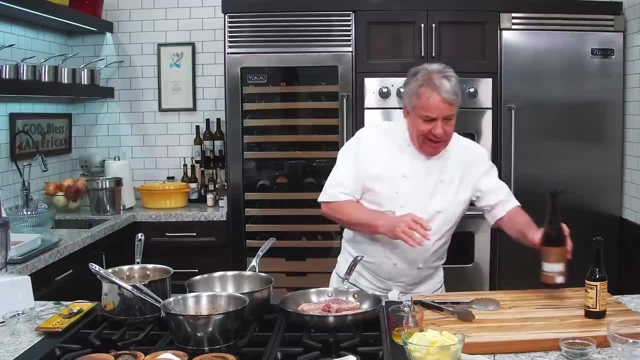 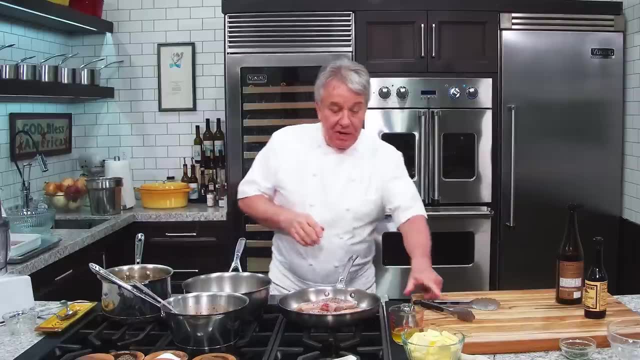 we're gonna put a touch of soy sauce- That's gonna be our salt- in there. okay, That's what we're gonna do. Really, really simple. If you have that porcini mushroom salt, you can put that in there. 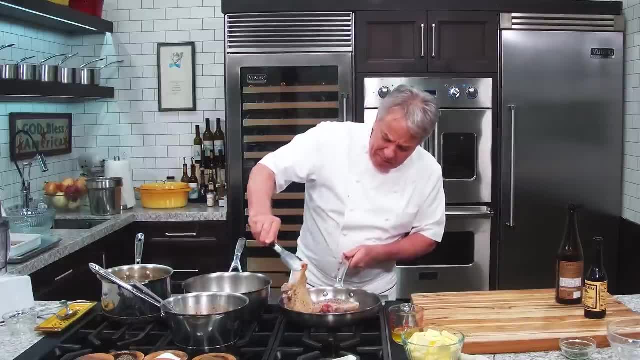 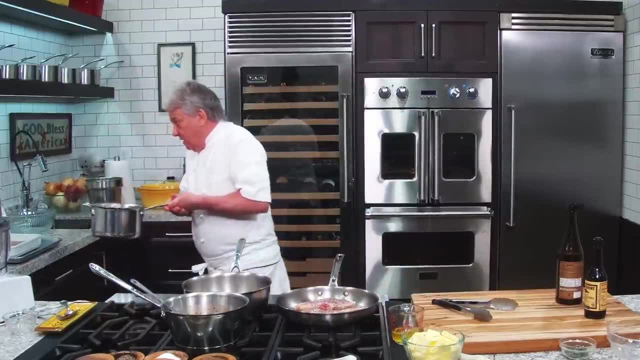 That would be actually very good. We're gonna wait until we have a better corn, And then we're gonna be doing fine, We'll reduce it a little bit. Let's take the potatoes. friends, The potatoes are cooked, Oh, I gotta show you. 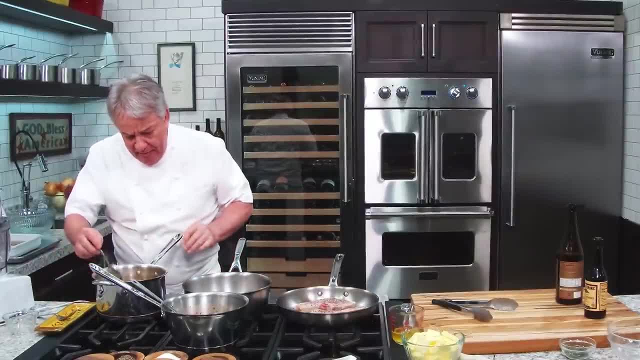 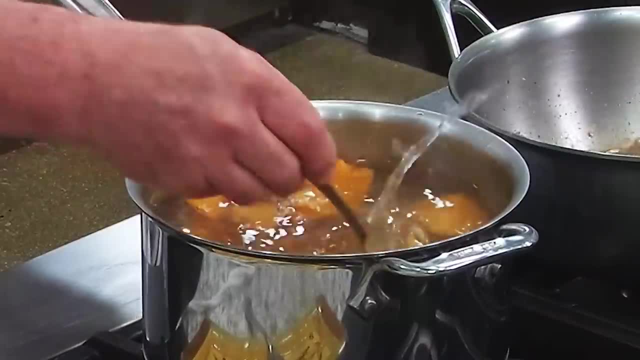 When I cook the potatoes, friends see, I put I shave ginger and I put whole garlic cloves in here. I can't see them, but they're in there. I put three whole big garlic cloves in there. Oh yeah, I found one. 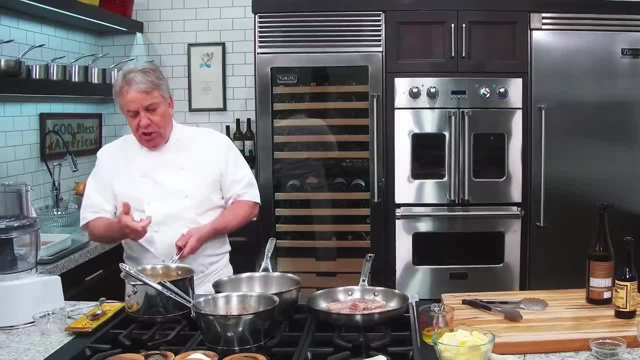 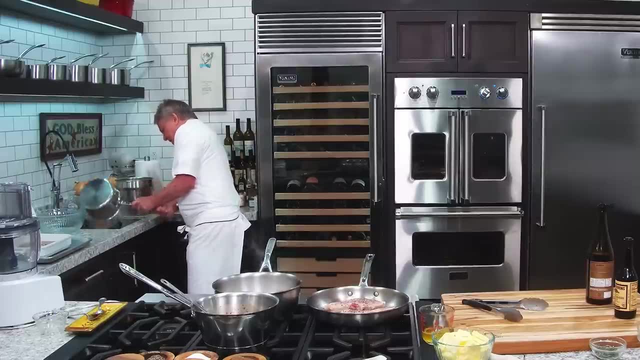 Anyway, it's in there, somewhere I put three garlic. this is two big potatoes. Two, two large potatoes, Two large potatoes. right, We're gonna strain them. We're gonna let them drain a little bit. See, the ginger is right there, friends. 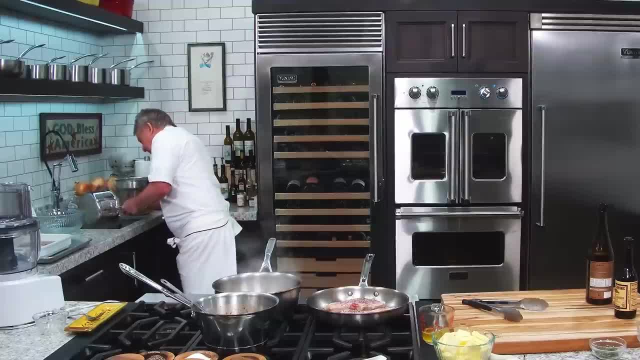 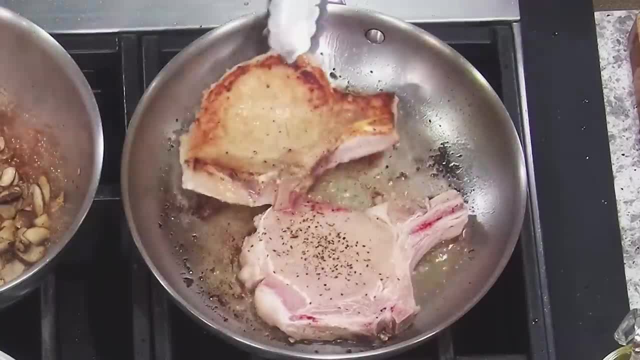 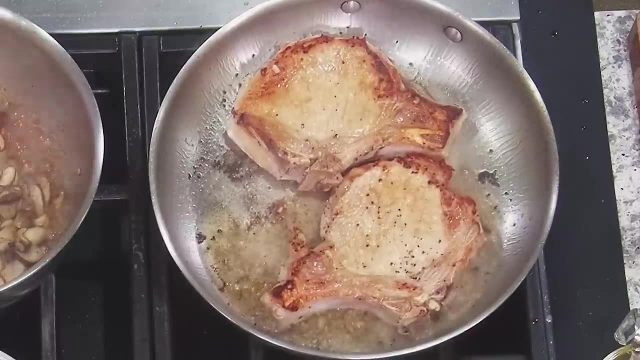 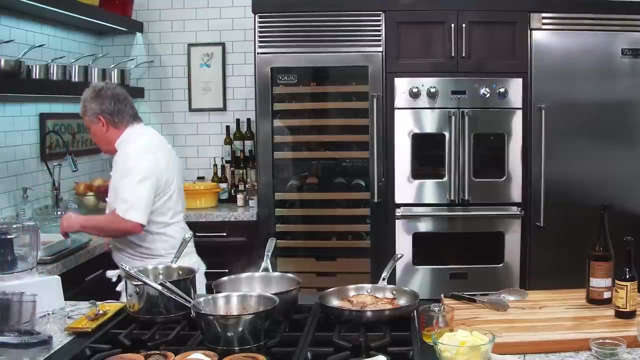 We're gonna take the ginger, put them right there. So the ginger and the garlic both poached. The ginger and the garlic, both are poached, which means then they are cooked and mild, especially garlic. We're gonna take it now, after it's drained. 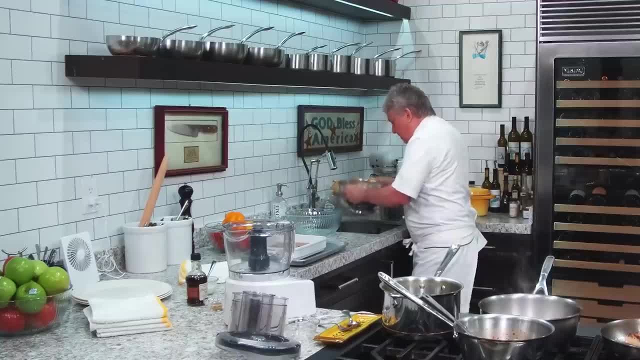 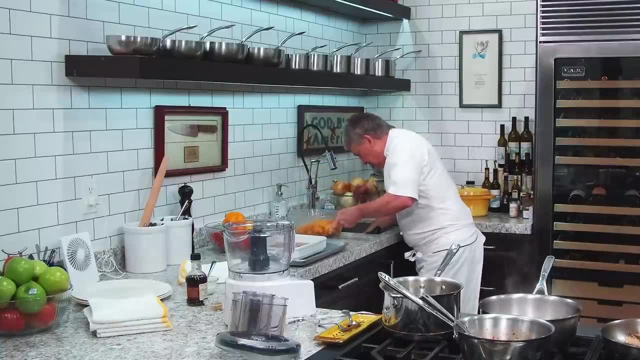 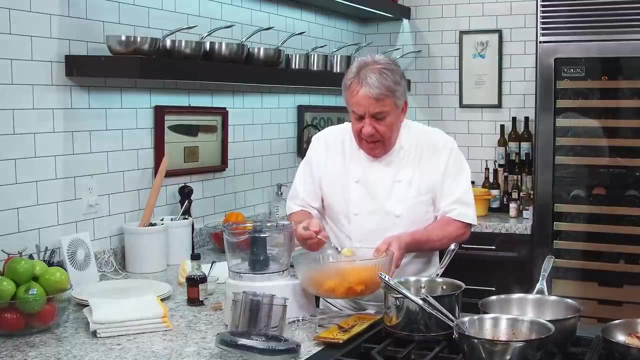 Make sure you take the time to drain them. really good, okay, I would probably take a little bit longer if I was not doing live TV. Oh, ginger, come back over here. you, There, you go. You see, look, Friends, you can see the garlic in there. 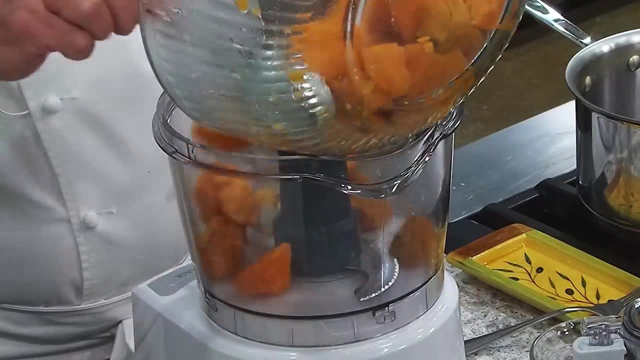 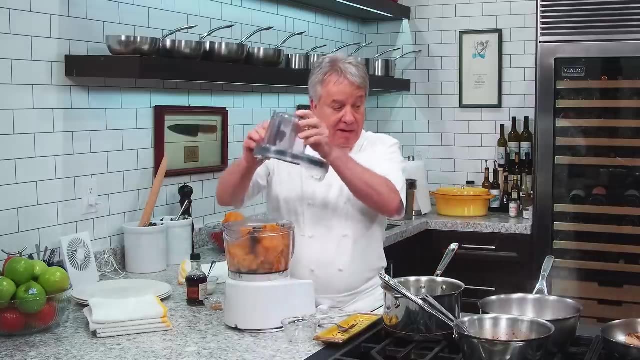 The ginger sliced it thin. We're gonna put them in here. I want you to take the time to drain them a little more. okay, But I didn't have much time because I'm doing so many things at the same time. Let me make sure we're doing well in here. 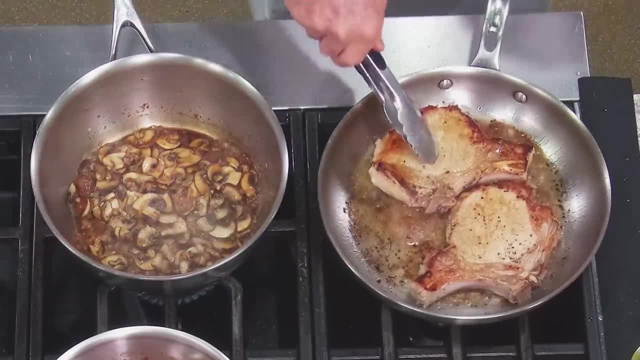 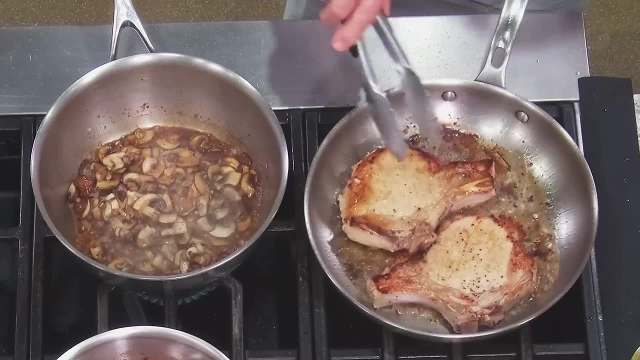 The sauce is very simple, right You notice? And those chops right there, friends, are gonna be just fine. We're just gonna let them rest, We're not even gonna put them in the oven, They're gonna be just fine. 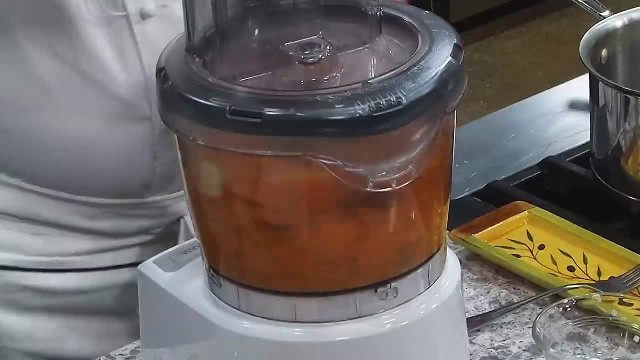 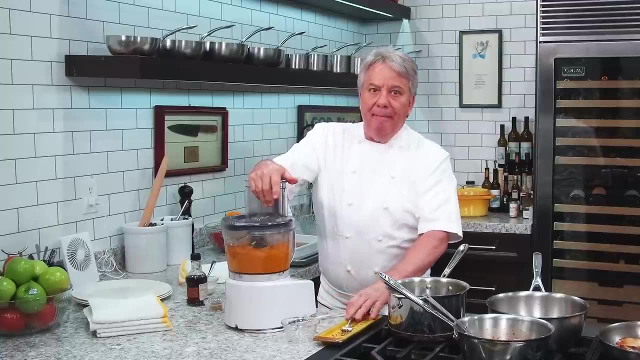 Gotta let them cook. let them cook. Okay, let's process the potatoes Now. you can't do that with regular potatoes, friends. Sweet potato's the only one. you can do that. Regular potatoes- they'll get gummy. 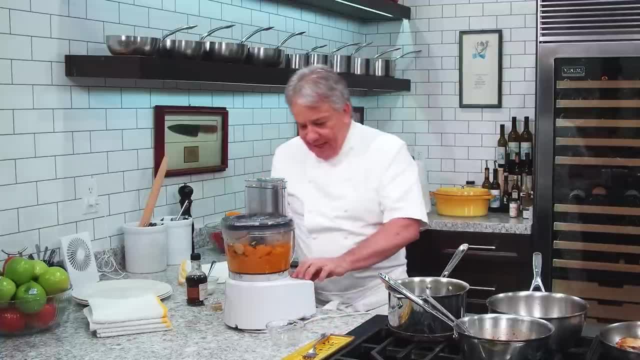 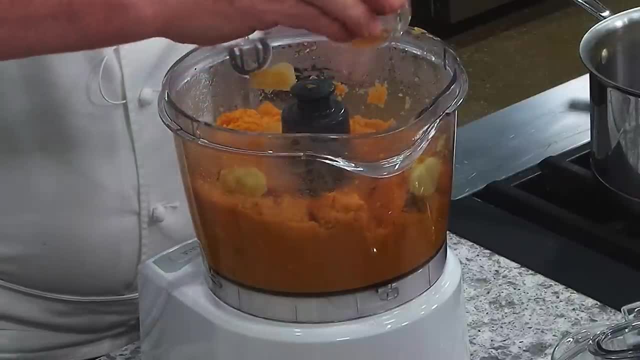 You don't want a gummy mashed potato, that's for sure. But the sweet potato they can take it. I'm gonna put a little bit of cumin- very little Cumin is wonderful folks, in a small, small dose. 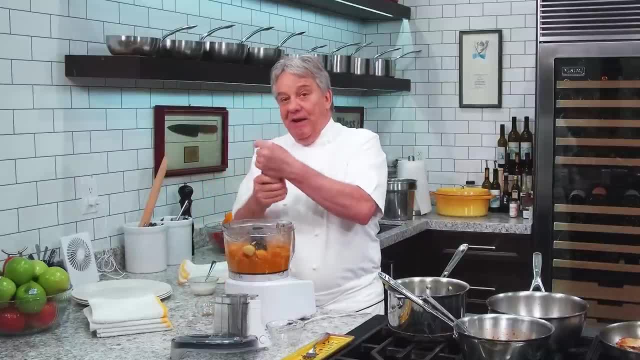 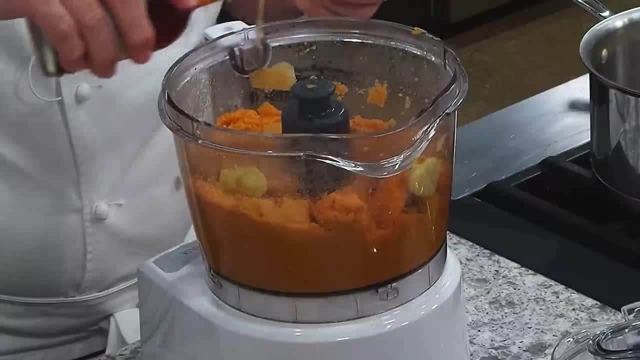 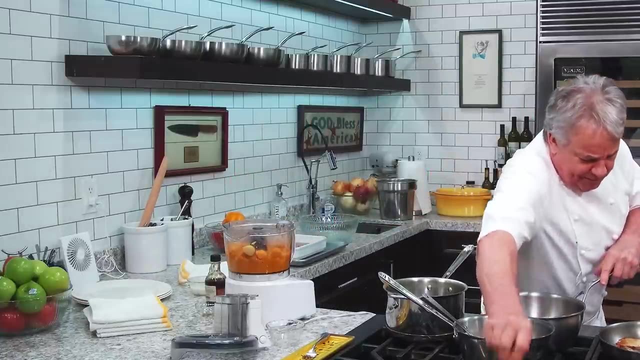 Very, very little cumin And a little bit of maple syrup. Oh wow, this is little maple syrup- I like very little maple syrup- And we're going to put a little bit of pepper. Everything is doing well. You know what I forgot? 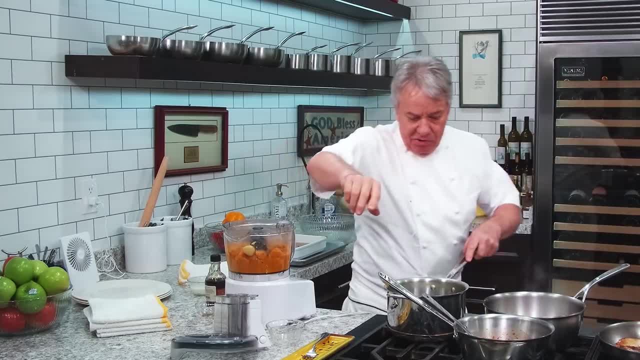 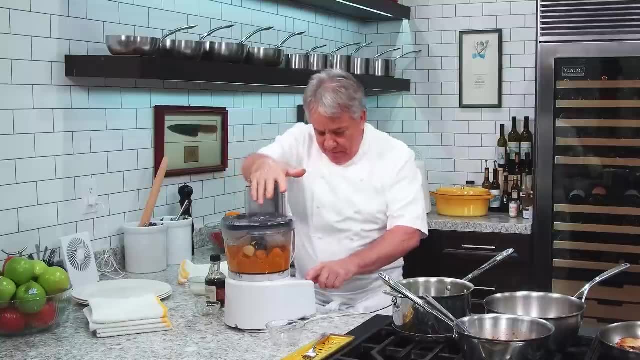 I forgot my marsala wine, But it's in my bar. I was wondering if somebody could get it for me, My marsala wine, Because I forget it. Here we go. I'll put a little marsala wine in that sauce, folks. 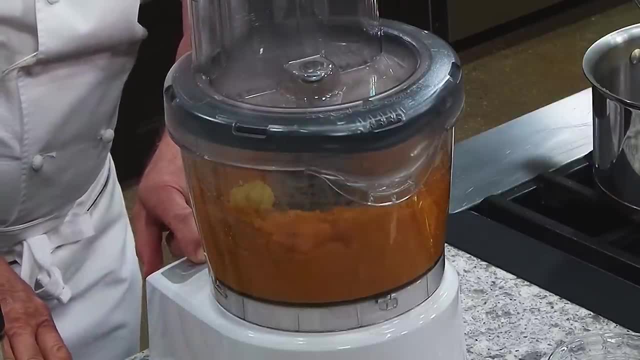 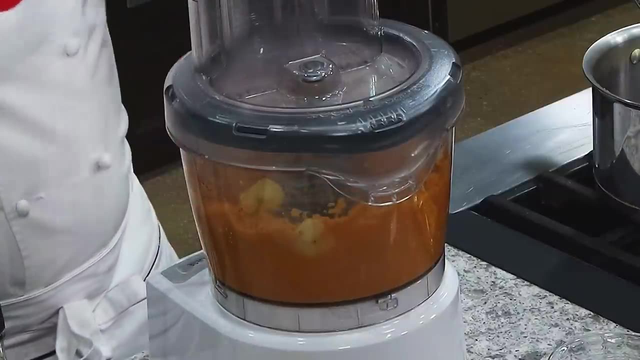 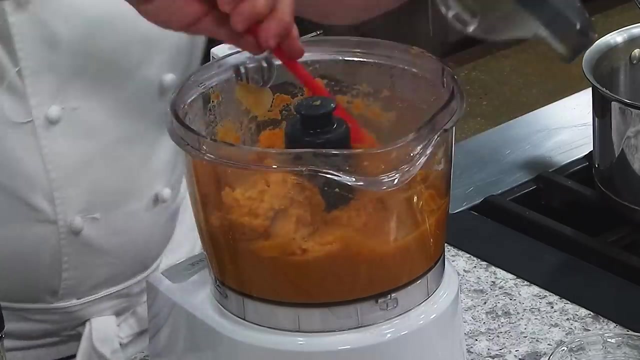 We're going to process those potatoes And hope that they get all mixed up pretty good. It looks good to me. Here you go. The marsala wine appears. That's great. I'm going to put a little bit of marsala wine. 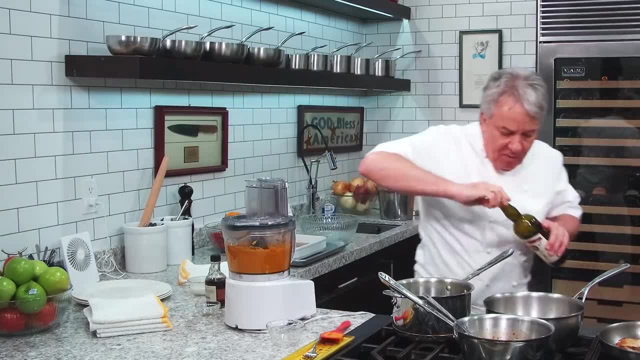 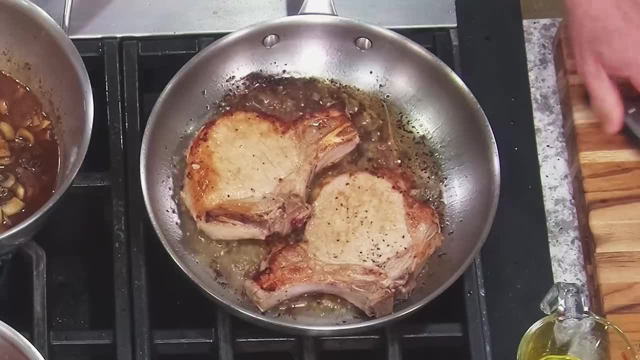 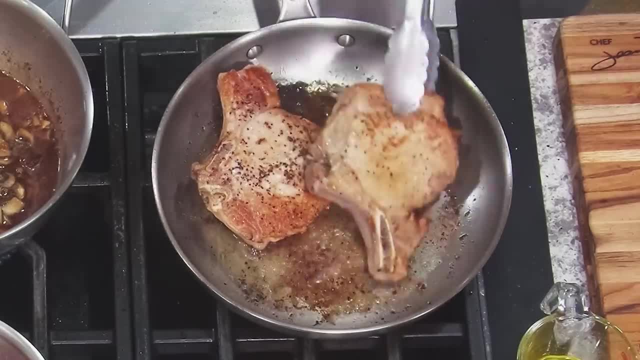 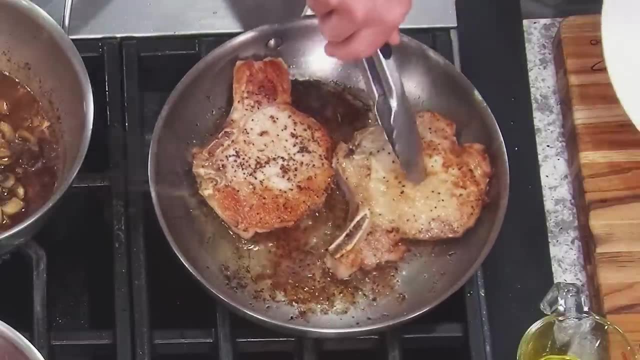 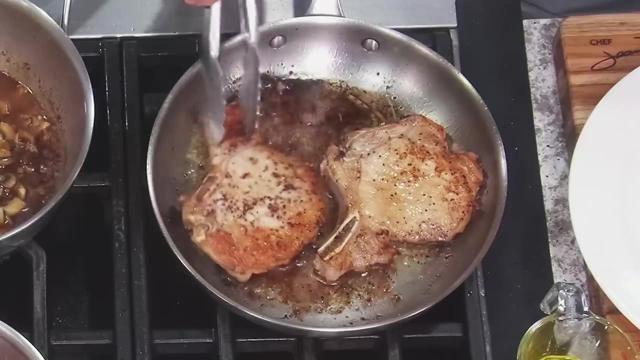 I'm going to take them out. friends, They're ready, Done. I'm going to take them out. I'm going to take them out. Let's see, Make sure They feel a little bit undercooked. You know what I'm going to do. 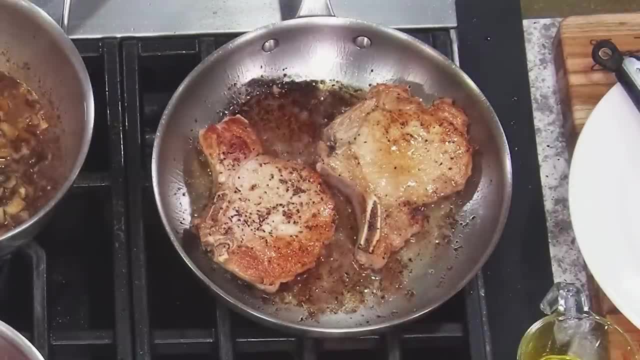 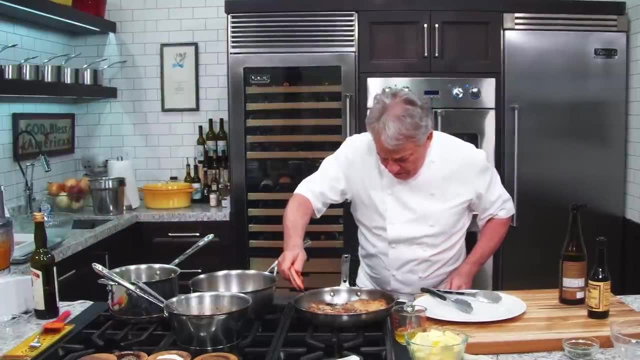 I'm going to do what I tell everybody to do: Check temperature. They feel pretty good. Those potatoes are done And let's check the temperature. friends, Let's see what we got. I think we can give them another minute or two. 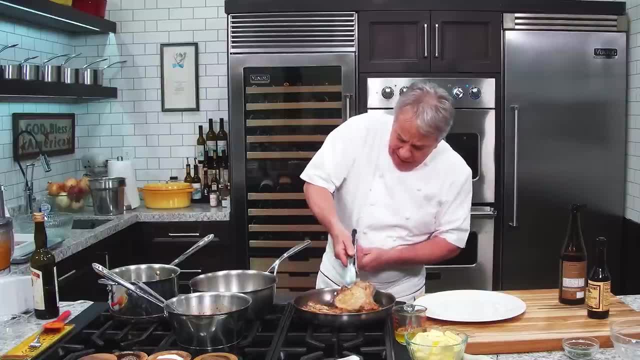 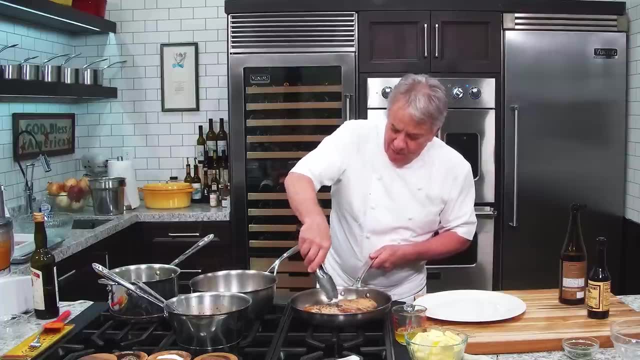 They felt a little rare at this point. still Now, as much as we don't want to undercook them, we don't want to overcook them either. I'm not worried about the bottom of it, because we're going to use that sauce, okay. 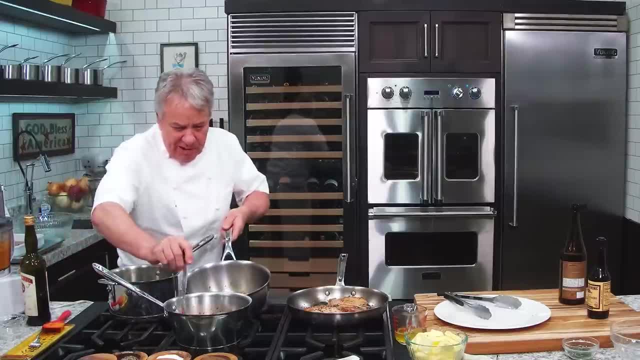 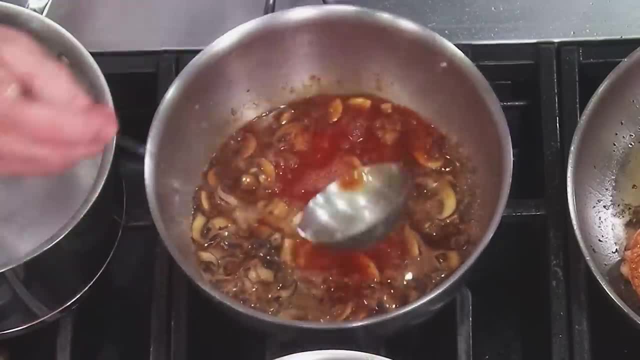 Okay, So did I put the masala in one? Yes, I did. Let me put a little stock in there, friends, Really simple sauce. eh, You know, I always forget something. right, I almost forgot the sage, But almost doesn't count. 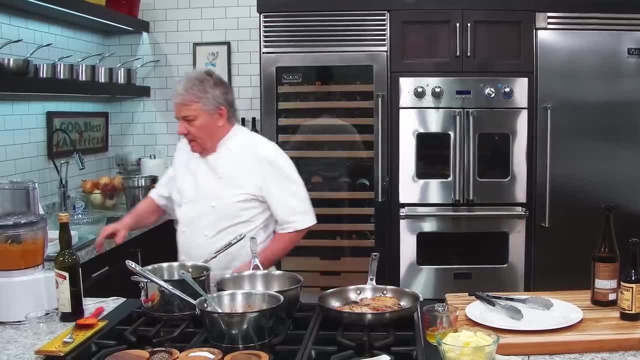 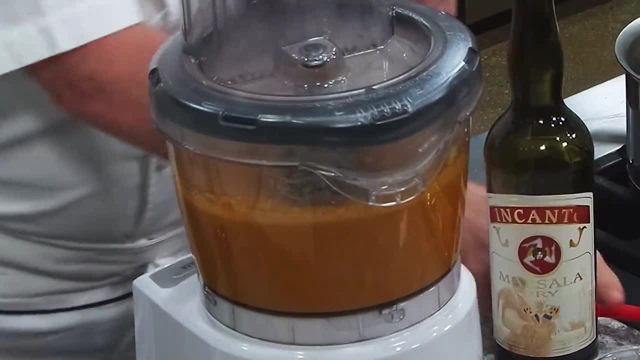 I'm looking. Did I forget anything? No, I didn't forget anything. Let's check the potatoes, Let's see what we got here. friends, A little smoother, A little smoother. Let me do a little smoother on the potatoes. 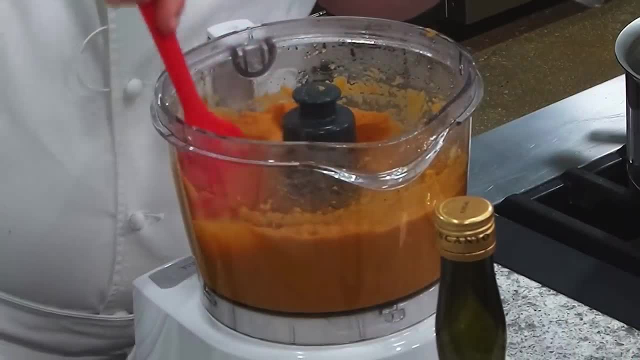 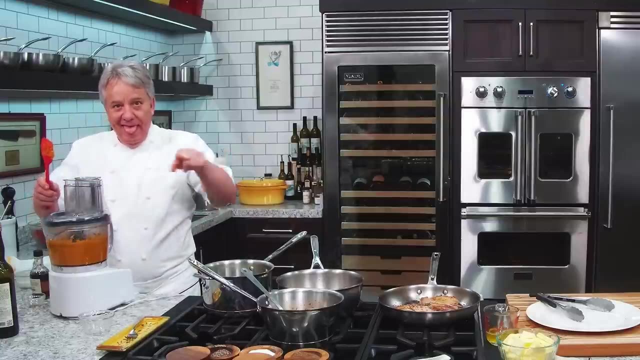 And I'm almost done, Yes, I'm almost done- A little smoother. And then you know what we're going to do: We're going to add butter. Yes, friends, we're going to add butter. All right, let's see. 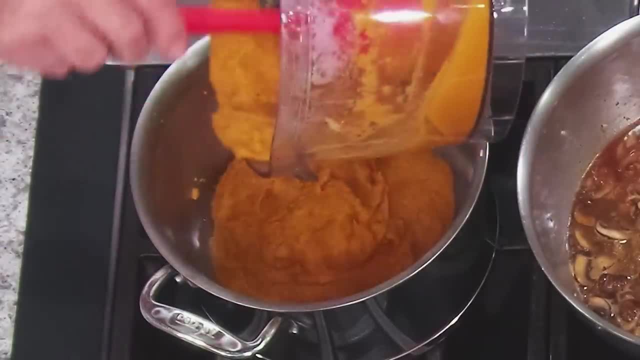 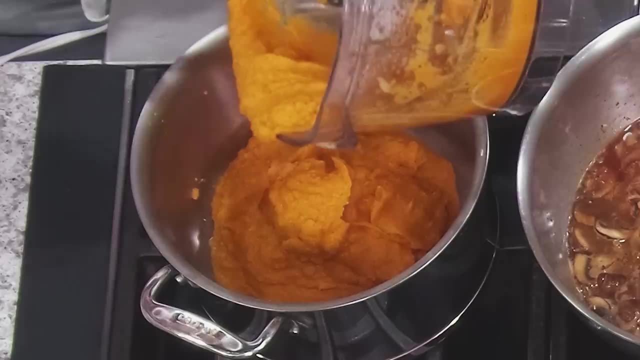 Oh yeah, But there's that down. See how simple that is. Now I do so many different things with sweet potato mash friends. We could do. we could add some corn in there. I saute some corn with onion and rosemary. 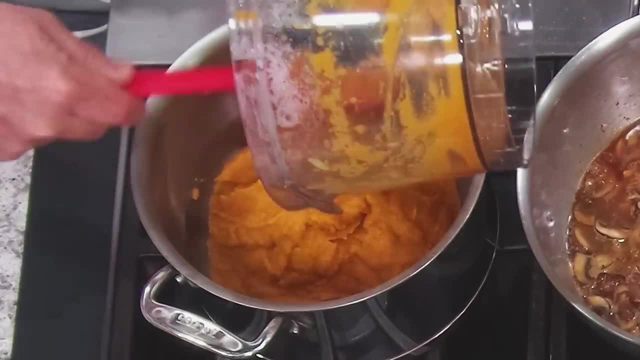 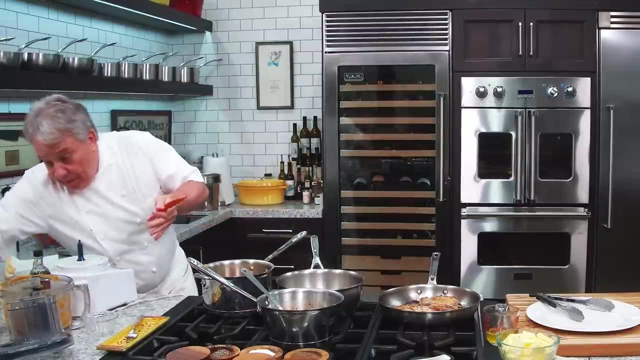 Sometimes I put it in there. You can do so many cool things with sweet potato mash, But this is a really simple, quick, easy recipe for you to do at home. Oh, mamma mia, There you go. And then all we need at this point, friends, is butter. 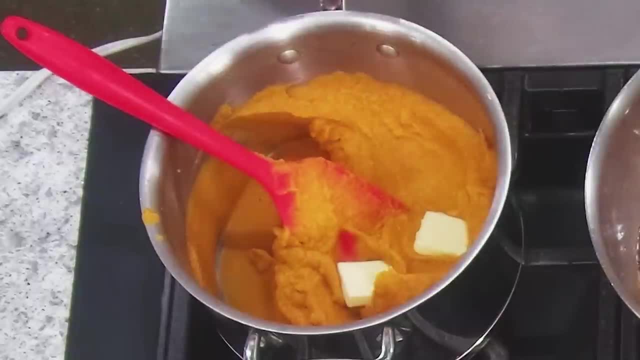 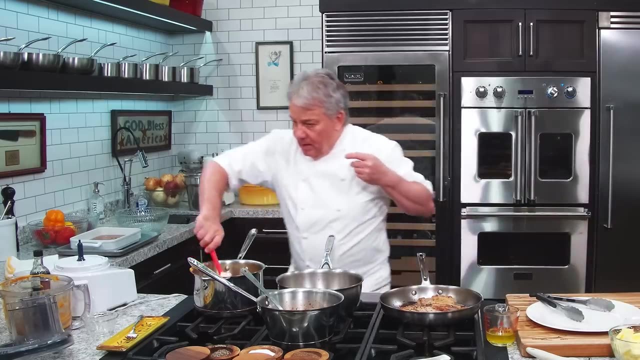 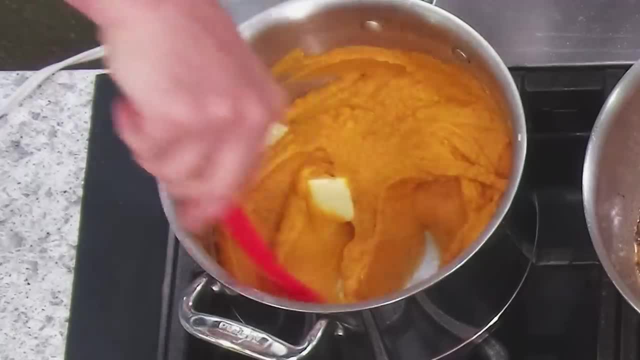 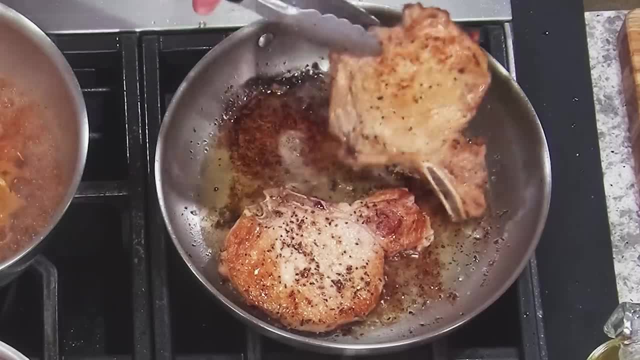 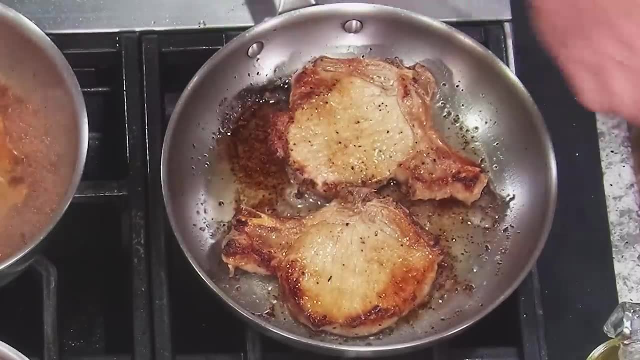 And here we have it. How are we doing on the food chop? Oh, this time they're down. This time they're down. I'm going to check them just in case. But I think they're down. Remember, don't be afraid to check them. 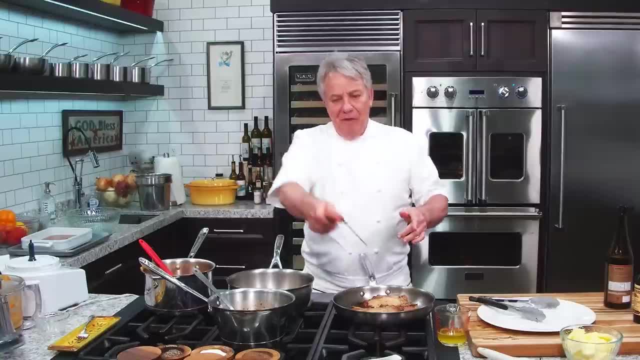 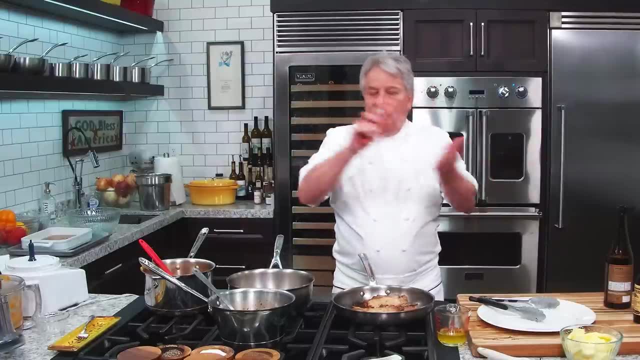 People say: oh, if you poke them, if you poke them, you're going to get a lot of butter him, you're going to release all the juices. that's so not true. if you're poking, you get just a little bit out where you poke, that's it. you're not getting all the juices out, you get just a little. 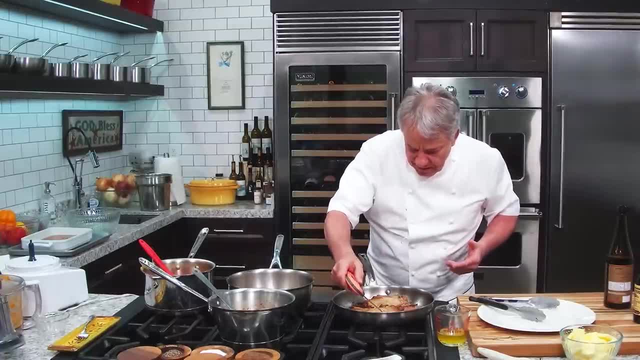 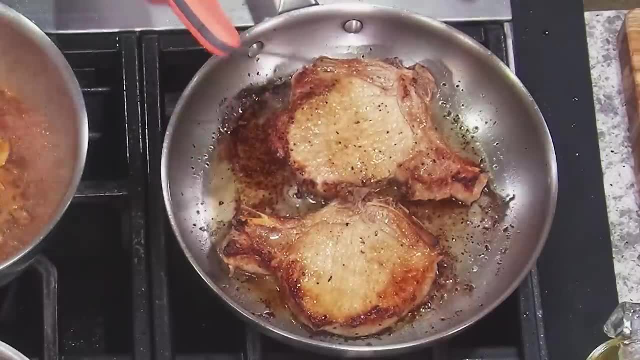 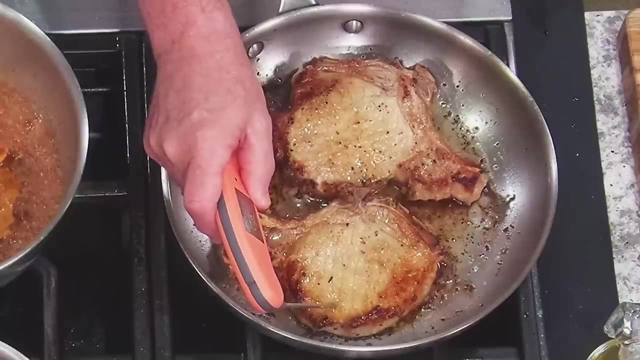 bit, so don't be afraid to poke. okay, you're not going to hurt him, all right, and i'm right now at about 125 friends, so we're still not ready. well, oh, this one, let me see. no, no, no, actually, i'm good, i'm good, i'm good, all right, we're gonna let him right there. we're good, let's turn him off. 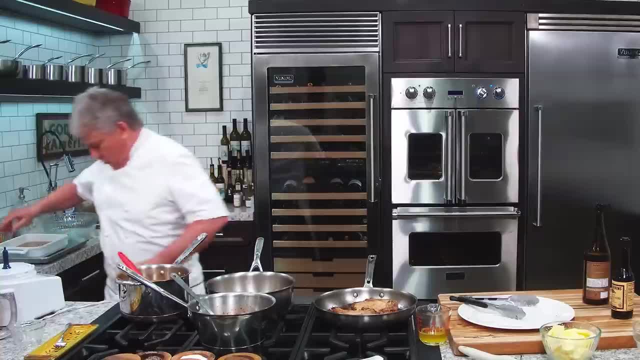 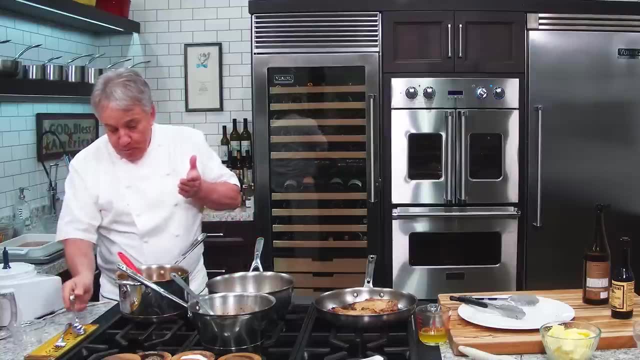 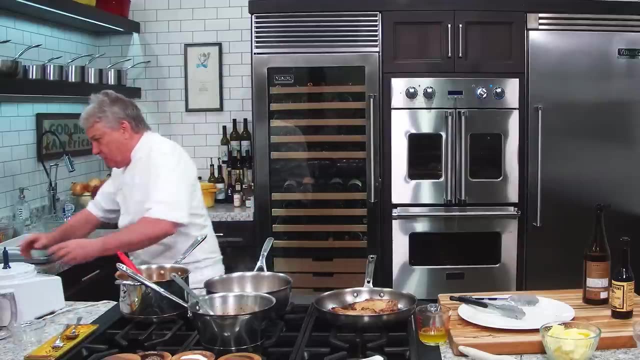 the mashed potatoes. let me test it, friends. let me make sure it's good. oh, i got my microphone while i let me check them to make sure they're good. they're delicious. the the sauce. we can certainly leave the sauce like that, but it's a little thin. 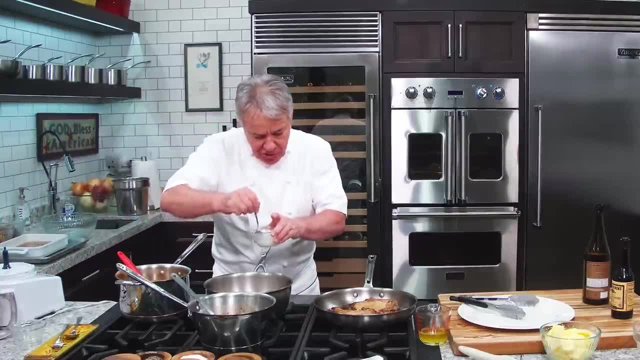 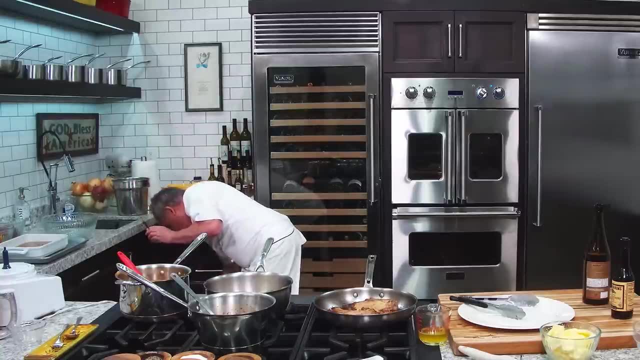 so you know what i like to do. a little bit of cornstarch, don't be shy. a little bit of cornstarch, it's not gonna hurt you. a little whisk would help the minute we put it in. we want to whisk it in the minute you put in your cornstarch. just make sure you're. 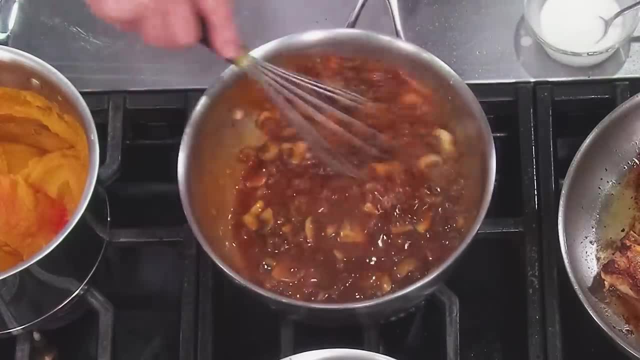 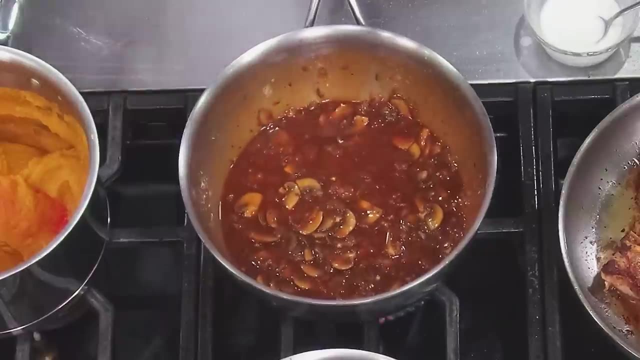 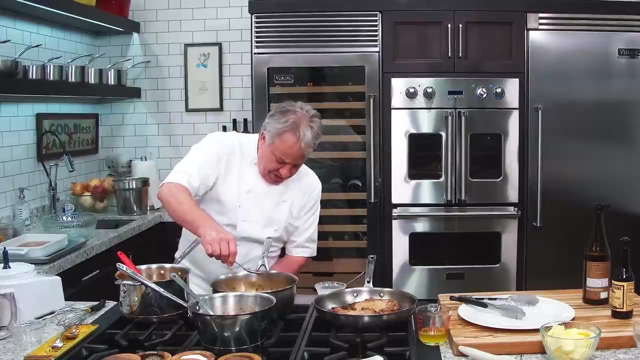 taking it. that's all you see. see how fast that went. holy moly. that smells amazing. the sage, the sauce. let me check it for salt. let me check it to make sure it's good for salt. friends, let me reduce the heat, i don't need that much. 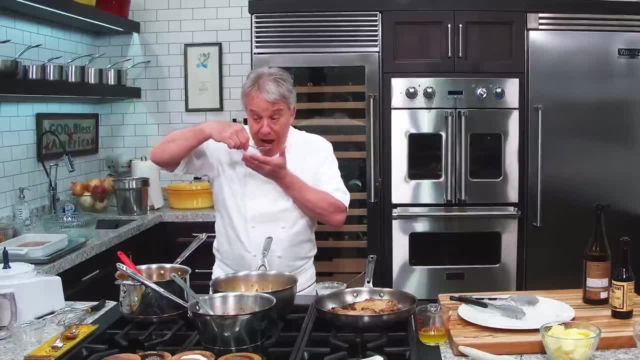 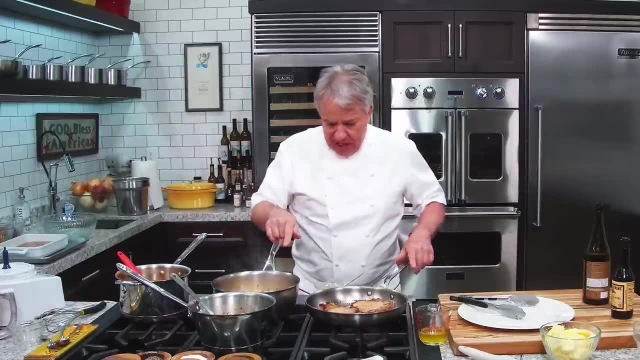 of heat. oh, this is hot. it's gonna be very hot. i gotta be careful. delicious as long as you like. sage that i don't. you could use taco, that'd be good. you know what could be good. also, in there is a little bit of cream. you could do that. you could add a little. 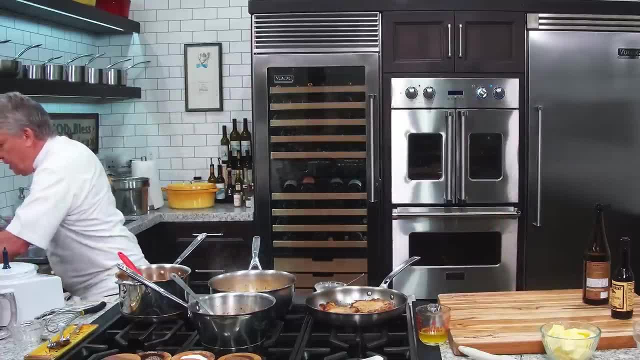 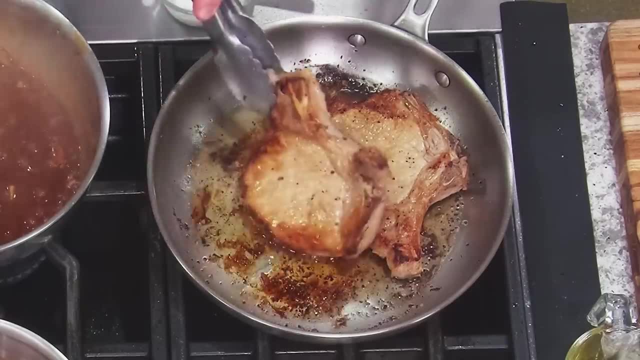 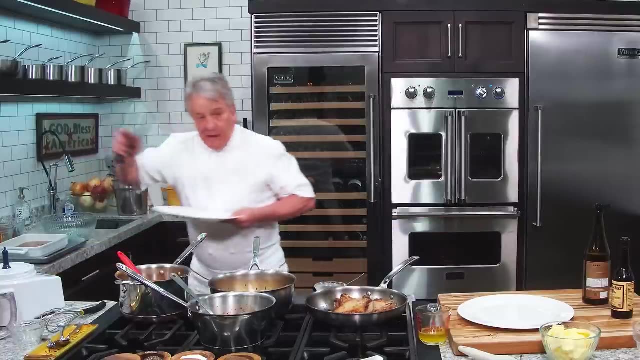 bit of cream. all right, friends, let me make a plate for dinner. let me make a plate for dinner. oh yeah, look at that. that's gorgeous. that's beautiful. now, what we could do also, friends, we could deglaze this. you know what let's do. it take a couple more minutes on the video, but i think 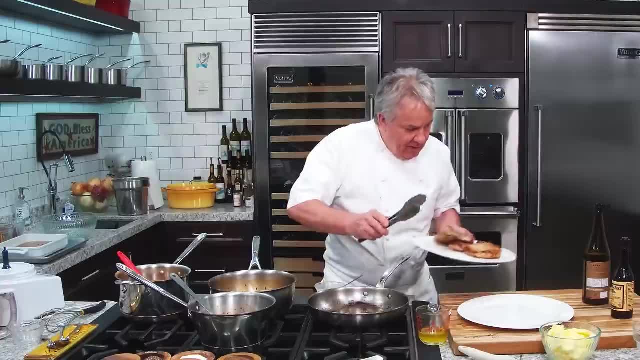 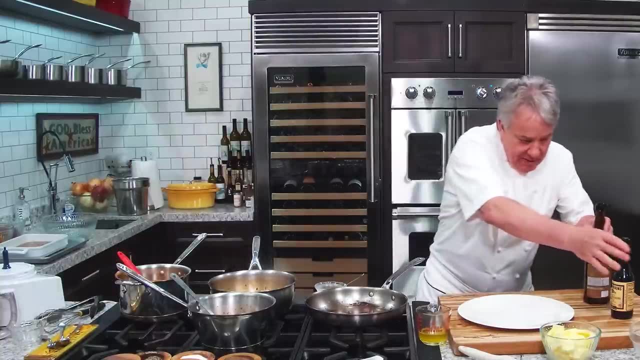 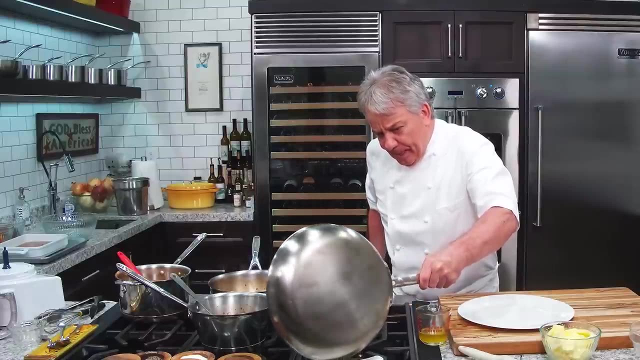 it's worth it. okay, now this right there, friends, we're gonna take them here, rest for a minute, stay here, don't go anywhere, and uh, what we're gonna do? we're gonna take the fat out of there. take the fat out and take a little bit. this is too good, too good. 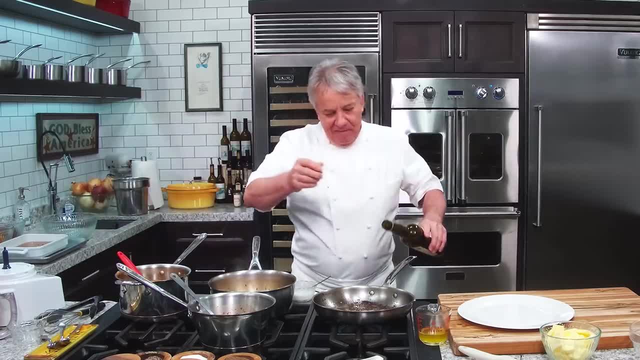 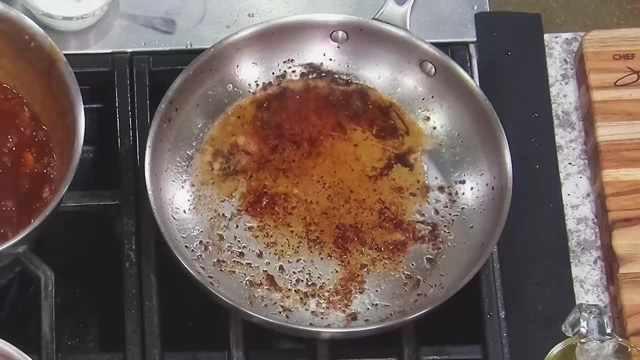 a little bit of fat, and then we're gonna take the fat out of there. and we're gonna take the fat out of there of the marsala, because, remember, marsala wine is one of those fortified wine that doesn't need to be reduced right. so that's the cool part. we can just do that you can use both: madeira, marsala. i. 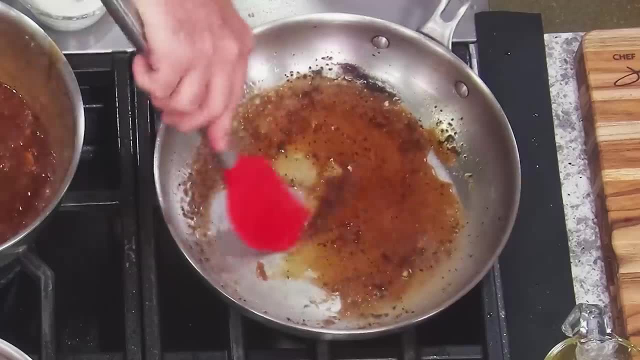 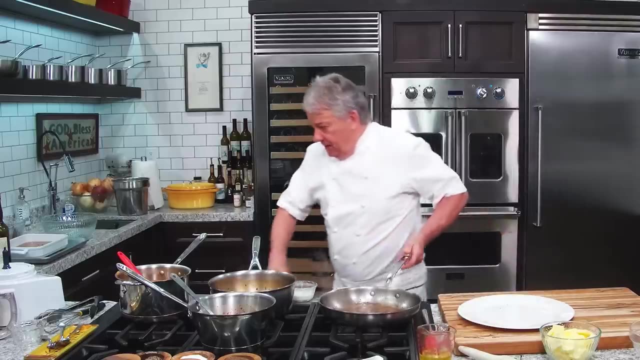 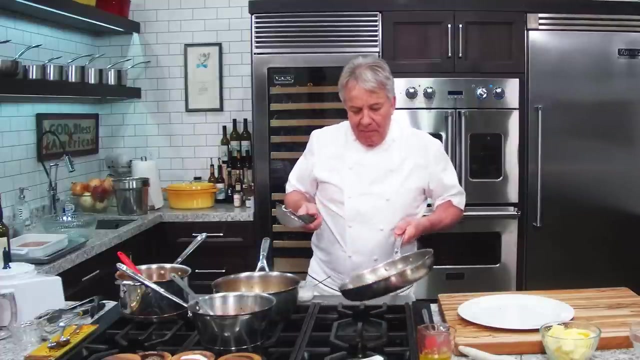 use them all the time because i love them. and now what i'm going to do? i'm going to put this, this fond deglazed, into my sauce. but, however, i'm not going to put this fond deglazed into my sauce. there's a little bit of burnt bits in there, so i'm not putting them. 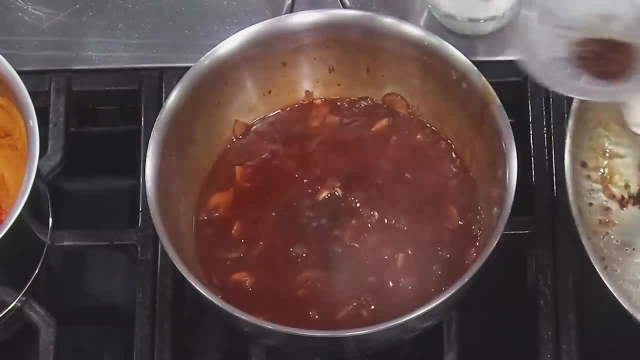 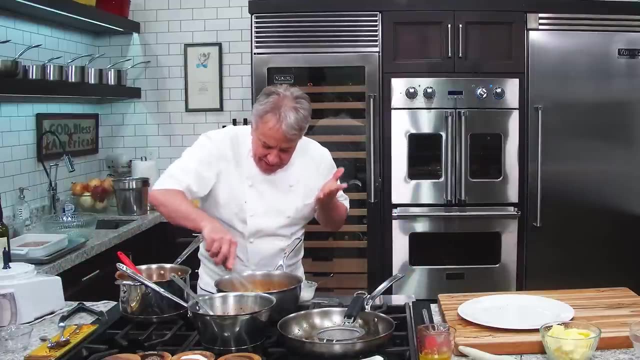 in there. that's why i'm straining them. see, straining them because i don't need the burnt bits right there. all i needed was a flavor. and guess what? right there, my friend, you have an amazing sauce and and the whole thing really took a little bit. i mean, it didn't take that long. 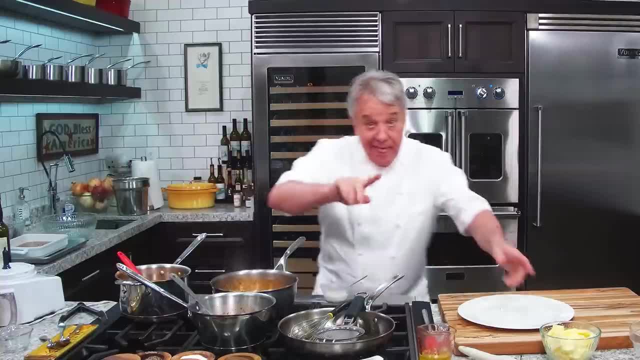 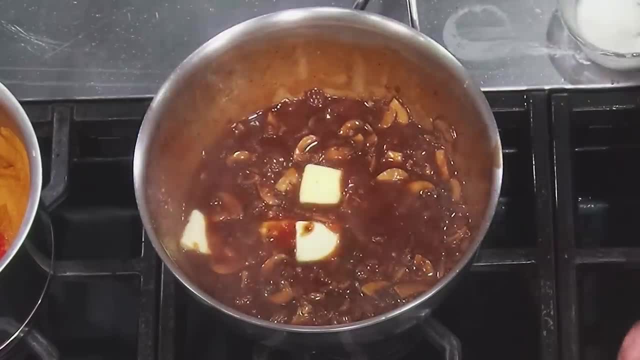 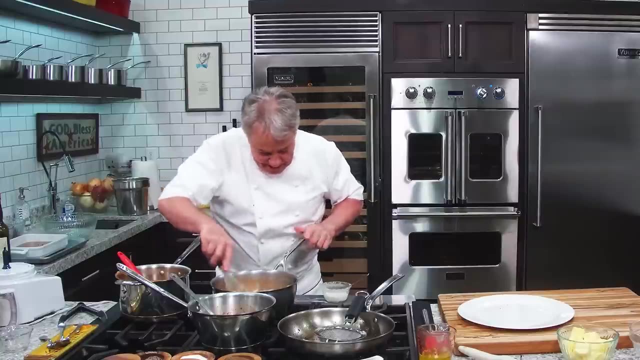 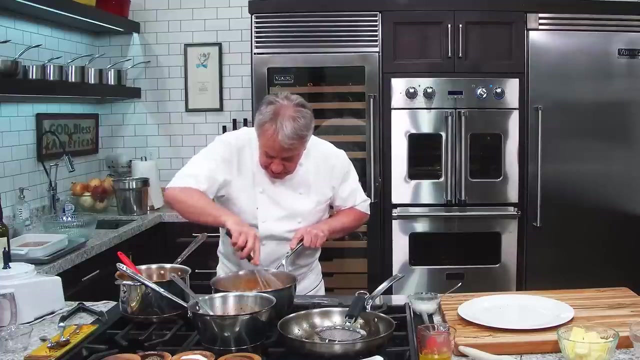 to do the whole thing and you know what would be good in that sauce. you said it. you're correct. don't be shy now. don't be shy. everybody loves butter. everybody loves butter. everything is better with butter, that's all. everything is better with butter. butter is the love of food. it makes everything good. you see, look at this, friends, now this. 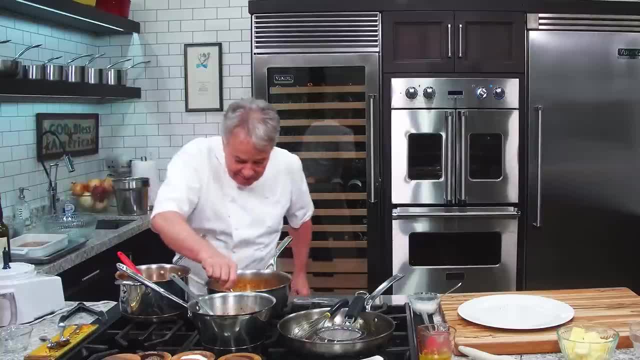 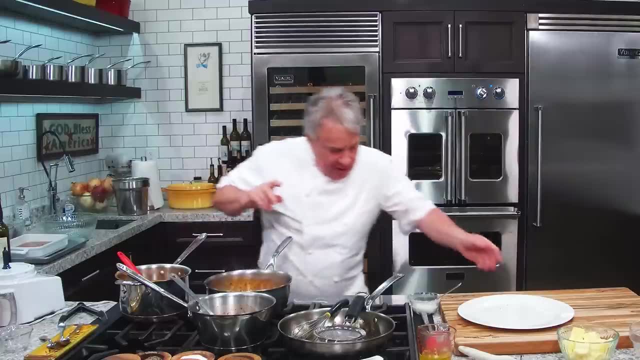 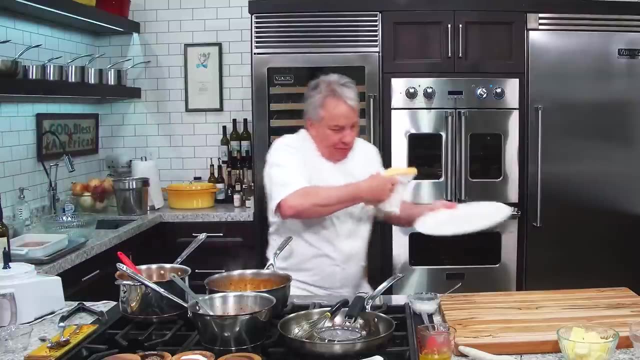 i gotta test it again. i'll test it again, friends, and let's see what do we got? okay, how do we plate this? do i have a clean plate? yeah, i got one right here. um, we're going to do this very simple, friends. all right, we're going to do this very simple. 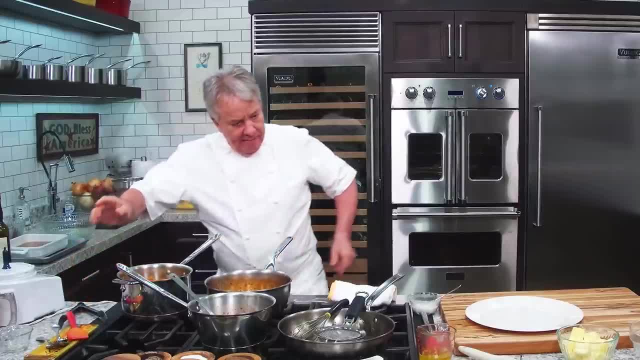 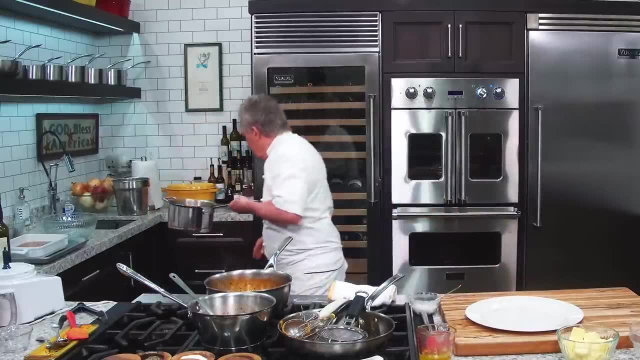 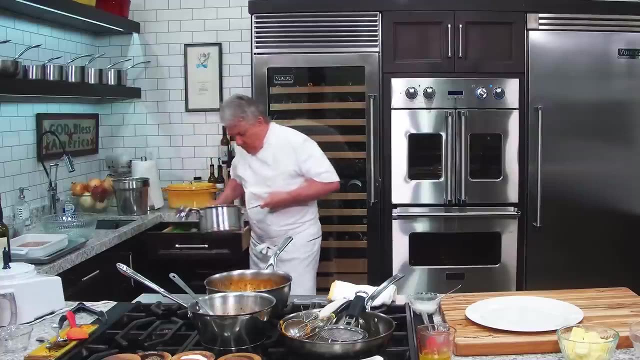 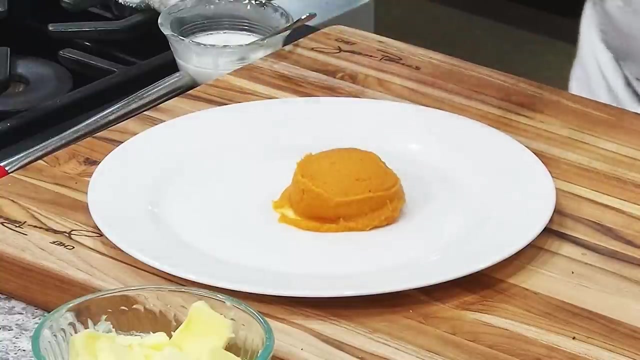 we're gonna take a ice cream scoop and we're going to put our mashed potatoes. it's not big enough. you need a big one, big, big scoop. i need my- uh, big mama scoop. I got to take in a spoon. it would have been the same deal. ready, same deal. 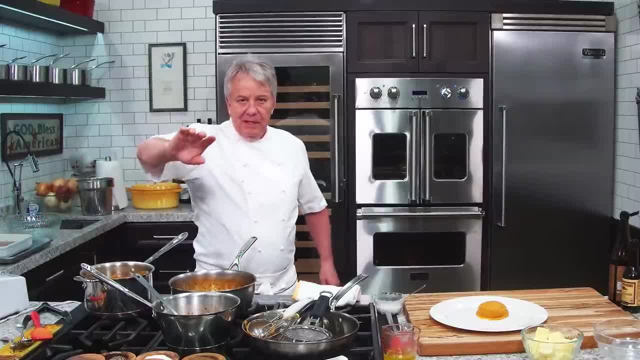 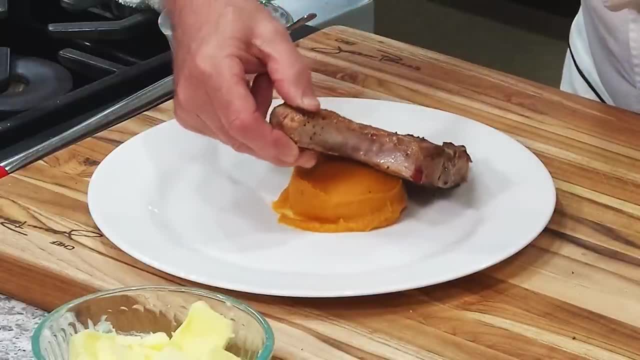 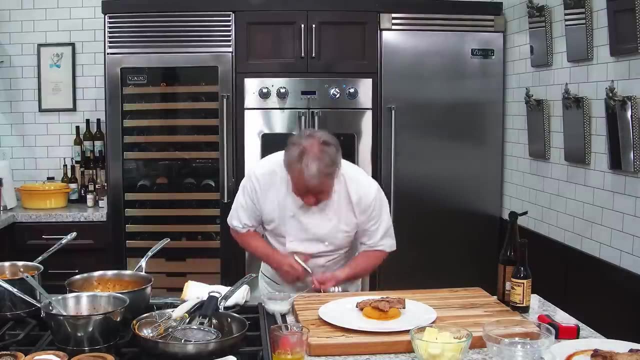 right there with a spoon. look at the mess I got. I got a mess in here today. why is my chop? let's put the chop in here, right there. very simple. then we take a little bit of that sauce right there and we're gonna put it. you know I. 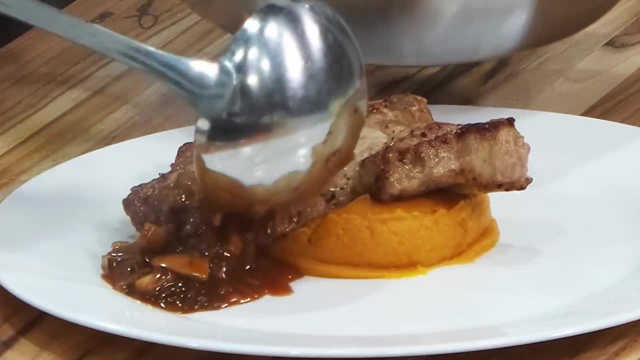 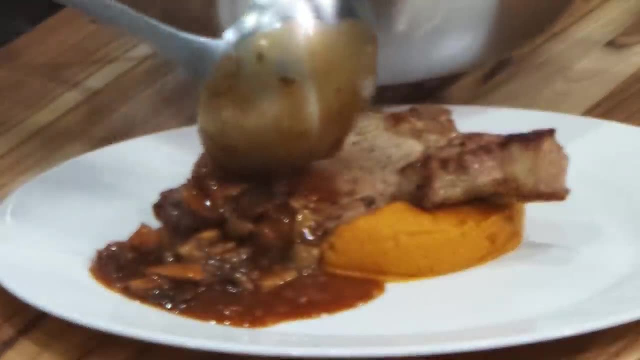 could have put some vegetables in there, friends, but I didn't have time to do this. you can certainly put the sauce all over the chop, but I think we're gonna be a little more elegant here and put a little bit on the side, and you know what.